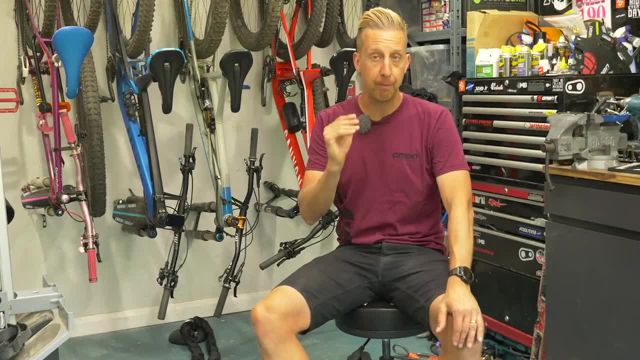 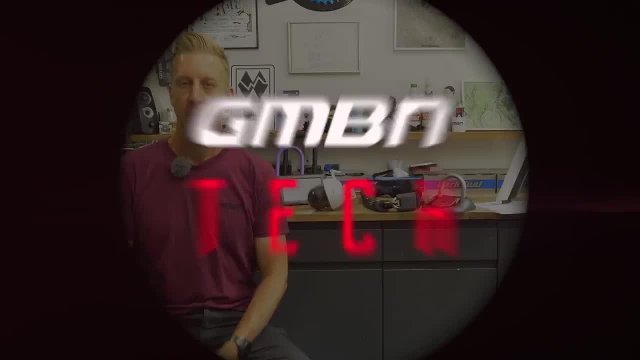 chucking it in a garage and closing the door. We're going to take you through some of the best security tips for keeping an eye on your pride and joy. There are a lot of different elements that go into keeping your bike safe and secure. I'm going to break this video down into a few. 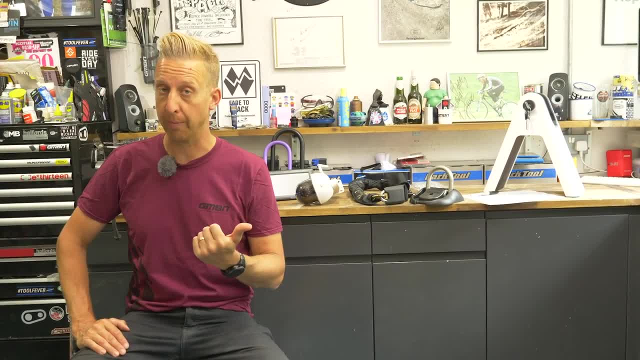 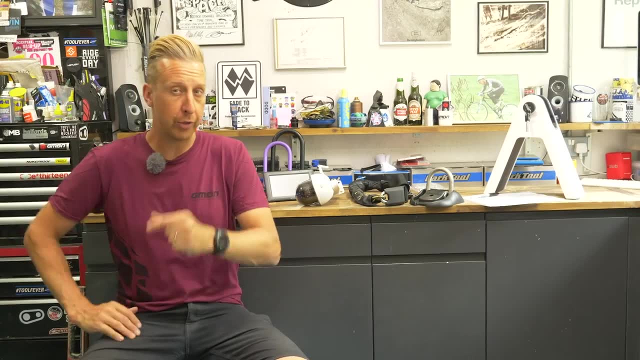 sections. It's going to include where you keep your bike and where you store your bike, how you lock your bike up and the things that you lock it up with, and then some additional protection and other things that you might not necessarily think of on a day-to-day basis. 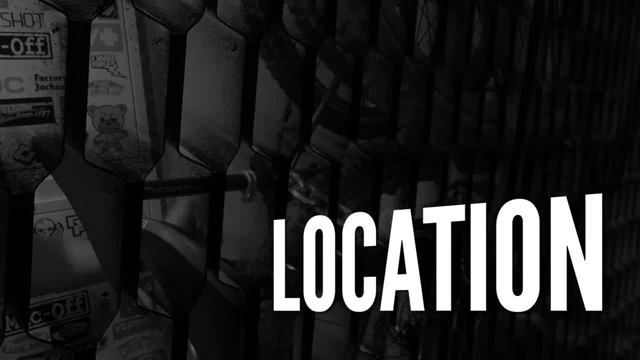 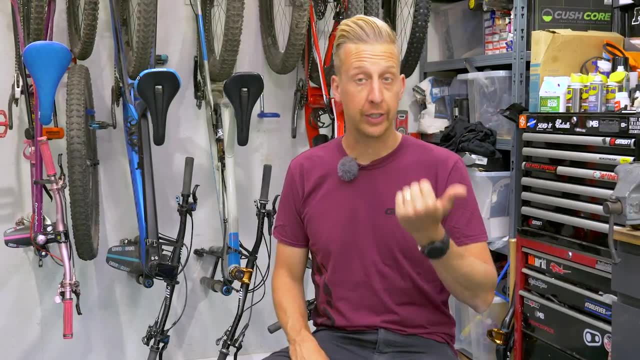 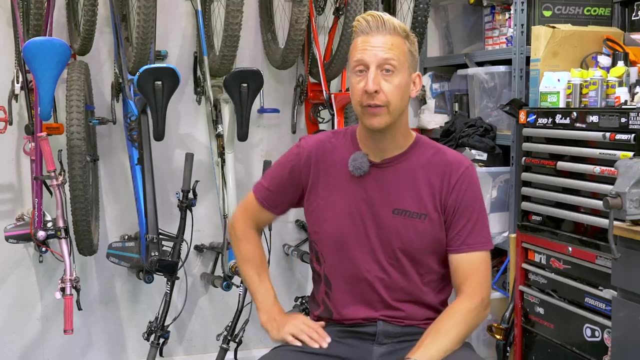 Let's start with where you keep your bikes. Depending on where you live, you're probably going to keep your bike either inside your house, in the garden, perhaps in a shop shed or some sort of outbuilding, in a garage or perhaps in some kind of workshop. 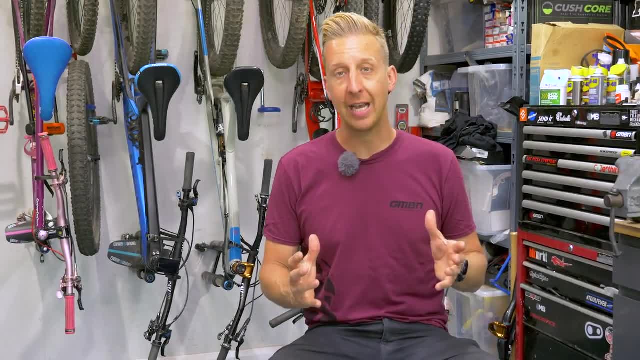 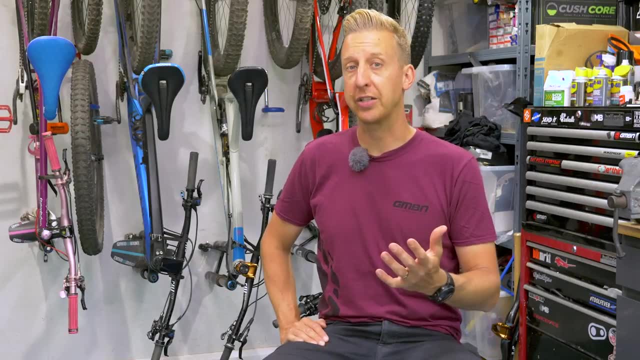 if you have something on the side of your house. Now, even if your bikes are kept inside your house, you're still at risk, because most bike crime is actually targeted. so that suggests that perhaps people follow you to where you live, or they know where you live, or things like that. 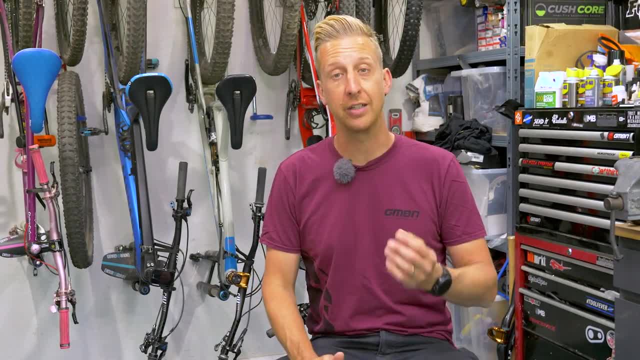 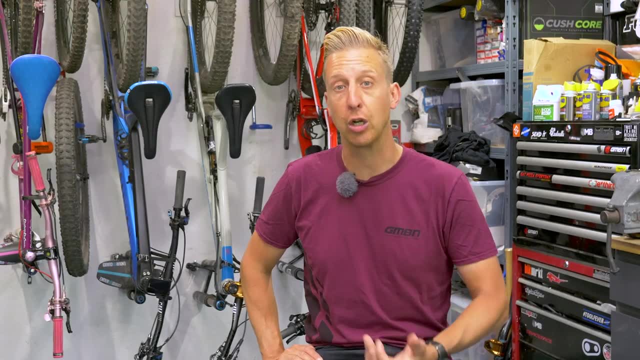 So it's up to you to make sure your house, or wherever you keep your bike, is as secure as it can possibly be. So with the basics, with a house, obviously it means having decent security on your house. That means good locks, modern locks on the front. 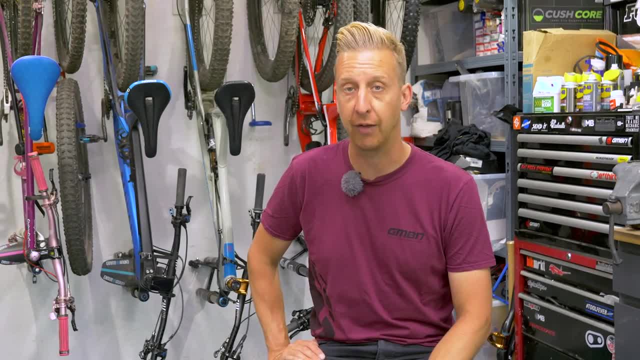 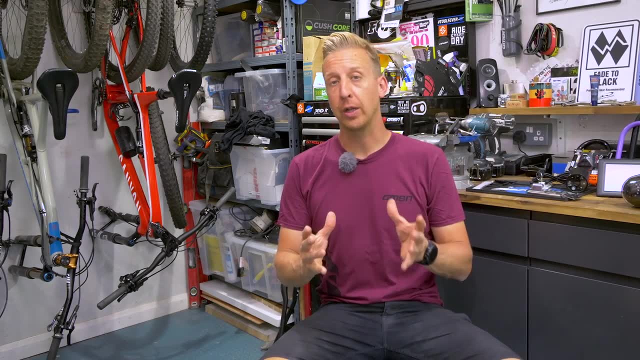 and back of the house. A house alarm is a great idea to have. And then, of course, you're gonna need things like insurance for your bikes, which we'll go into a little bit later in the video. Now, if you keep your bike in the garage outside, 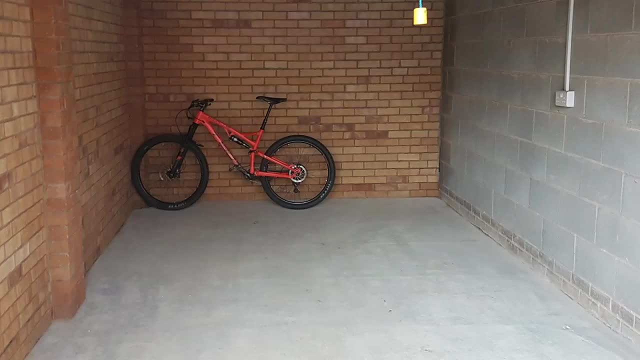 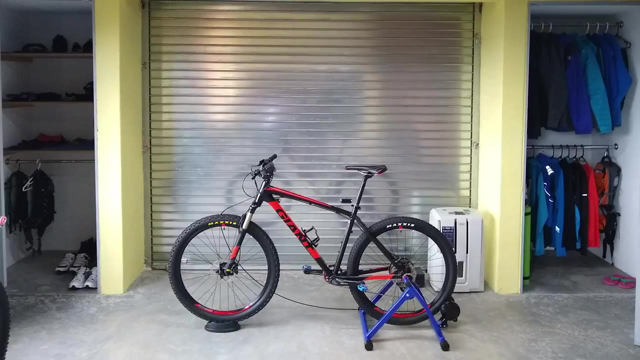 then there's a few things you need to take into account. Obviously, a concrete building is gonna be fairly secure, but the weak point is gonna be the door, So you need to make sure your door is strong. it has a good lock on it. 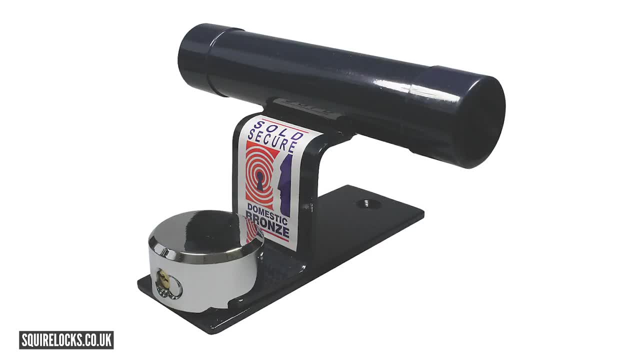 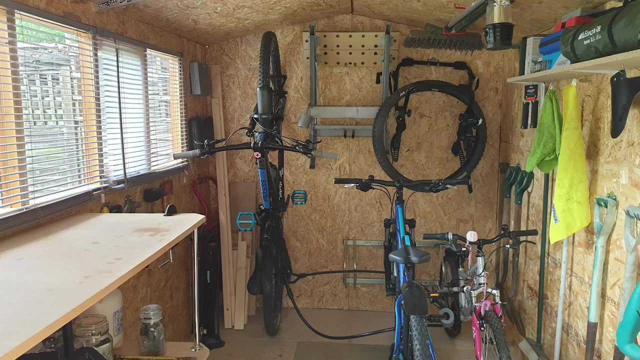 and it's definitely worth considering having a garage door defender. Now, a defender is a kind of additional lock to mean that the door can't actually open. Now, many mountain bikers use the common garden shed to keep their bikes in. This is absolutely fine if you have a secure garden. 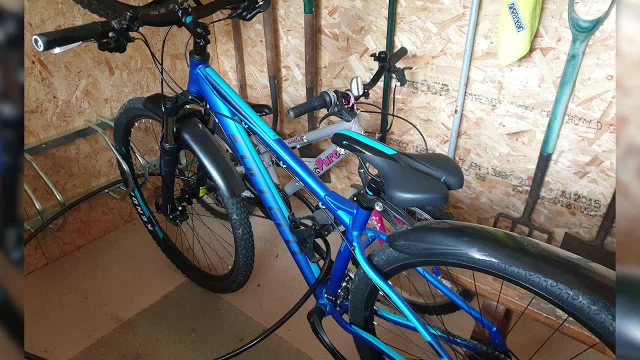 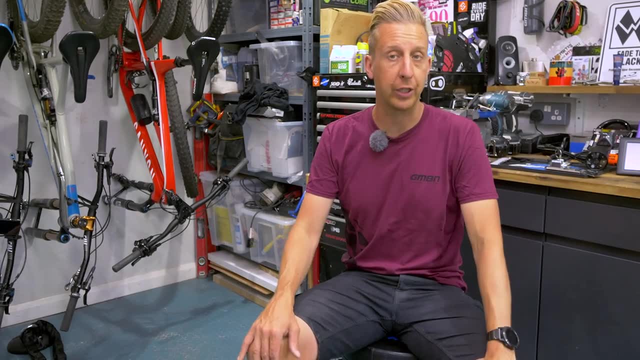 because most likely people would have to come through your house in order to get there. But if you have any sort of side access or any way that people can get into your garden, then you definitely need to make sure your shed is really, really secure. 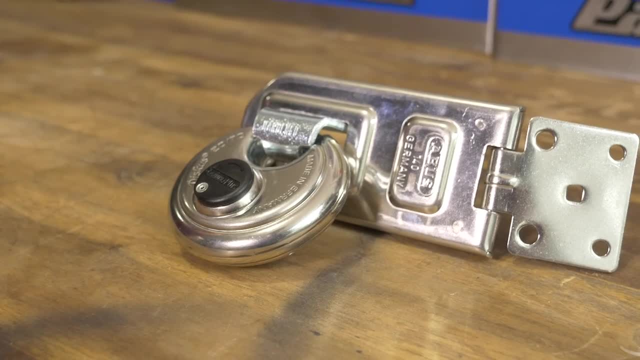 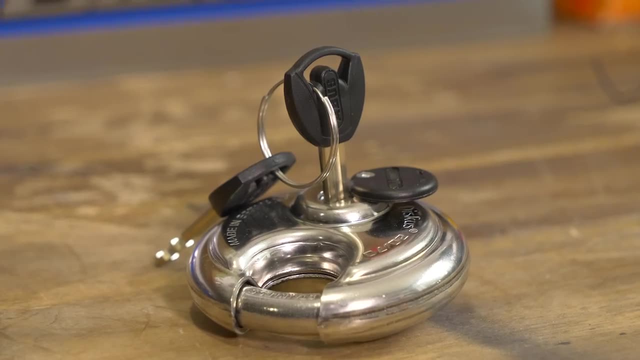 So you're gonna have some decent sort of shed locks on there, something like this: a quality disc style lock. It's not gonna corrode when you leave it outside in the garden and the key, the mechanism works really well. But more importantly, you really should have 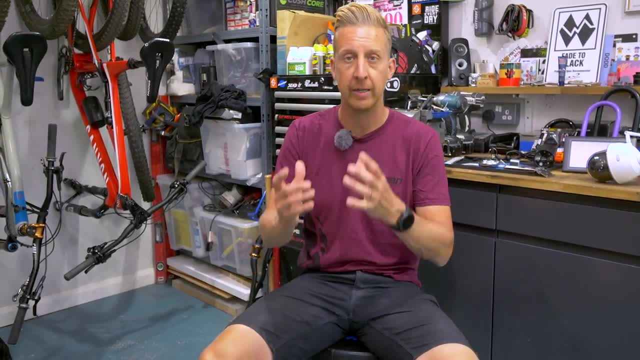 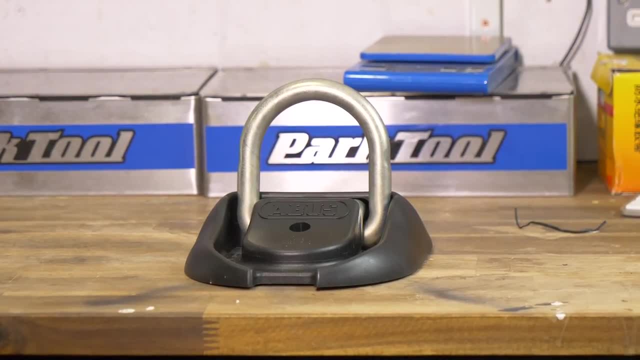 an anchor point in there, something to lock the bikes to something solid like a purpose built ground anchor. If you're gonna have one of these in the shed in the outside, then you really need to have a concrete base. These are designed to be used outside and inside. 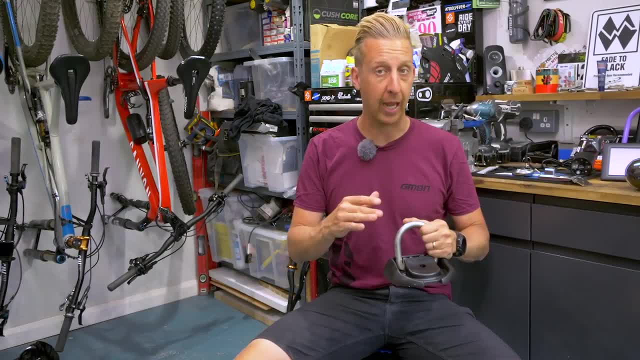 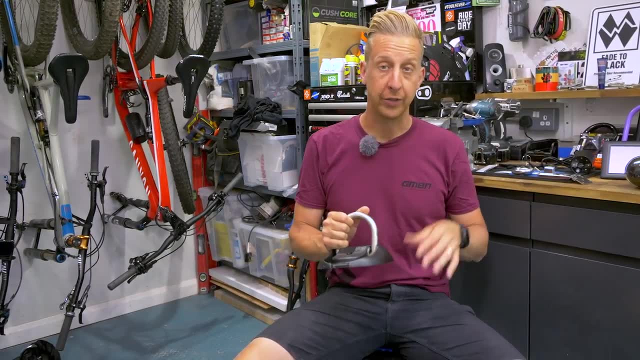 They're corrosion resistant, and once you've got them, once you fit them, you can pretty much forget about them. So it would be perfectly acceptable to lock your bike to one of these, and then you could have some kind of shelter over your bike. 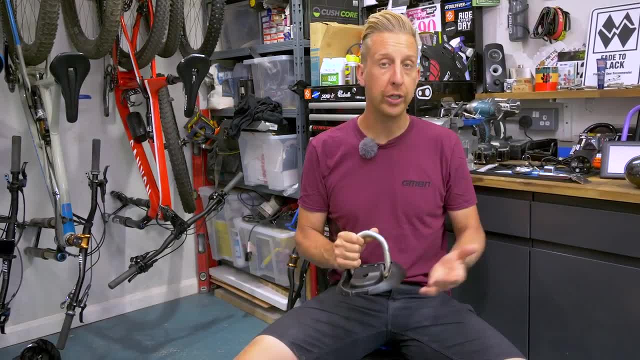 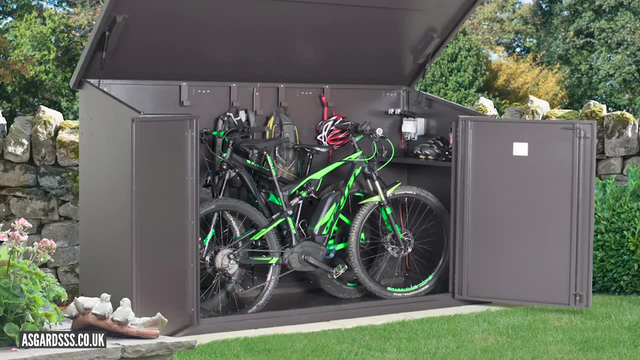 So you could just have a sheet to keep the moisture away from your bike, or you could go to Whole Hog and get yourself a dedicated bike storage unit. So these can be in the form of metal cupboards and metal lockers. There's a company called Asgard that make 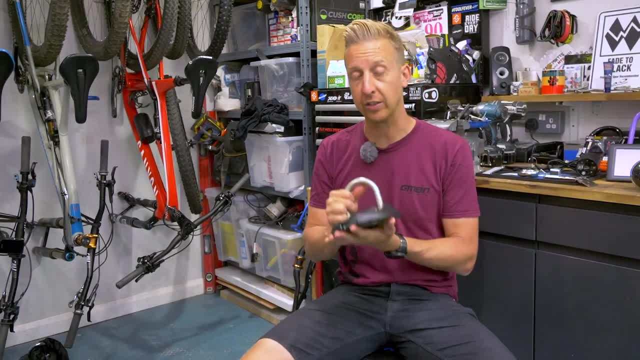 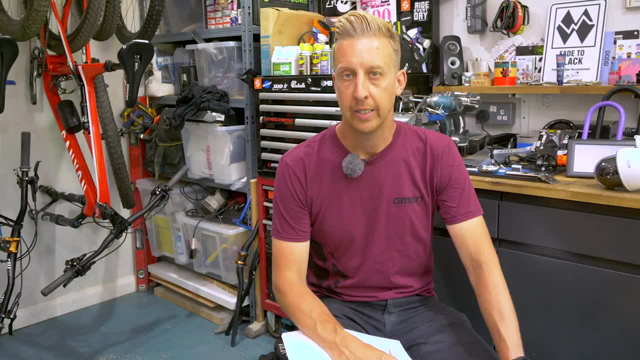 really industrially strong ones. They're compatible with things like ground anchors. You can even get ones that have got electricity points in there for charging e-bikes and your bike lights and things like that. Now, whilst your bikes can be locked up and safe, 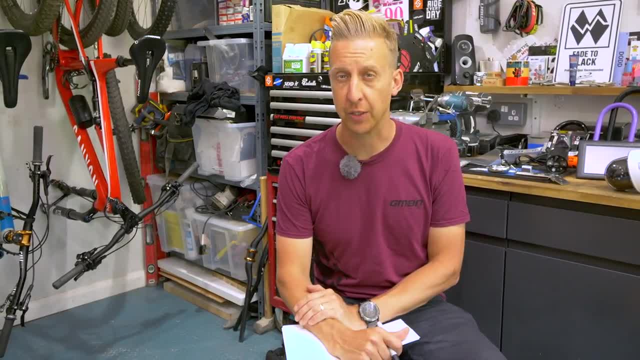 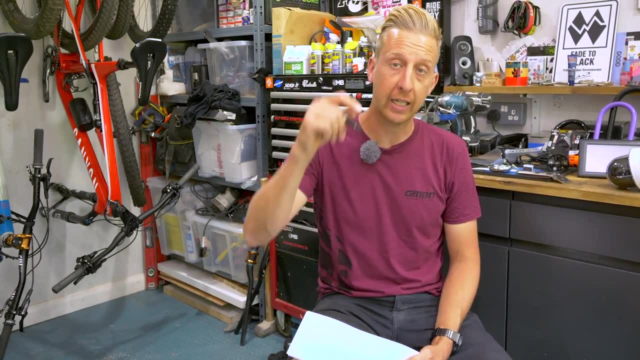 on the inside of your house, it doesn't necessarily mean your house is safe. So something actually quite nasty to talk about is a thing called the Thieves Code. Now, if you want to learn more about this, I'm putting a link underneath this video to Abbas Cycling. 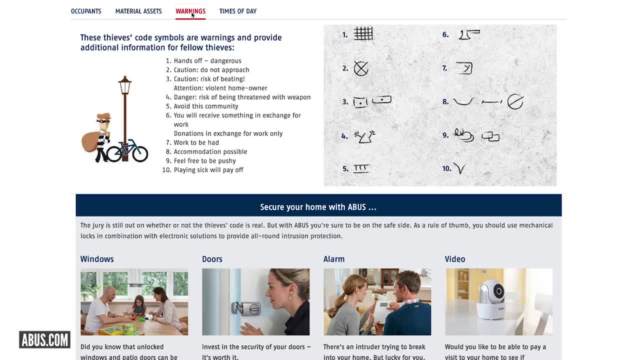 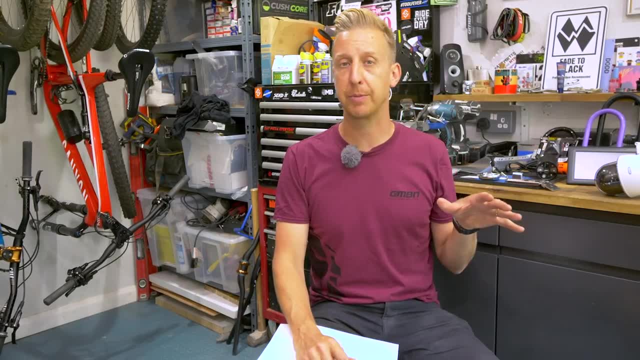 So that is the German manufacturer of locks and all things bike security. They've written a whole article about the Thieves Code, so I suggest you read that. But what is the Thieves Code? Let's just put this into perspective. You might be coming home from a riding trip with your mates. 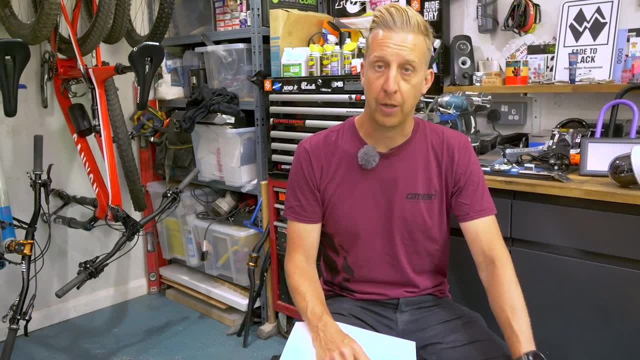 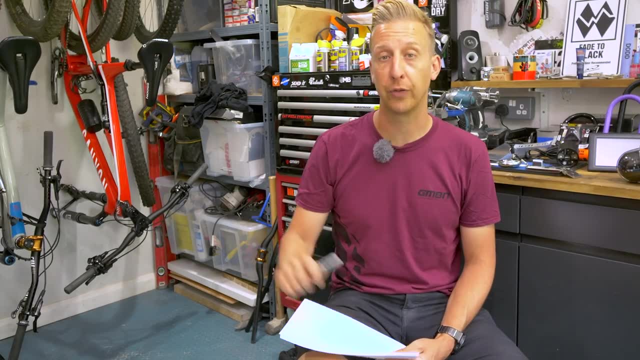 and you don't realize that you've been followed by someone in a car. Now that person will note where you live and then they might make some kind of marking on the outside of your house for another thief or another person to come back and then later. 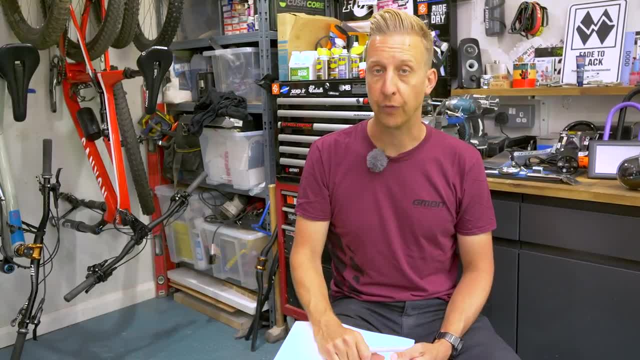 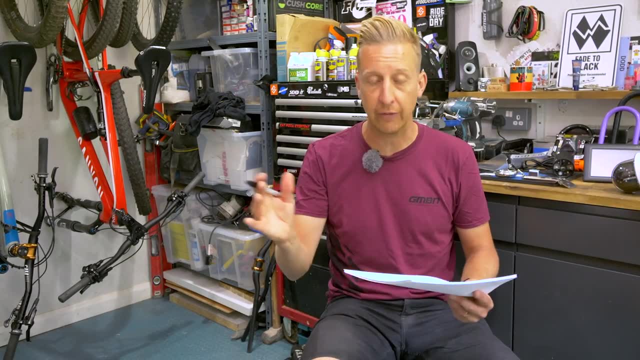 correlate that to which house it is that has the bikes in and then let themselves in and nick your stuff. Now this is also something to do with organized crime. There's loads of different sort of acronyms and hieroglyphics and codes and stuff that they use. 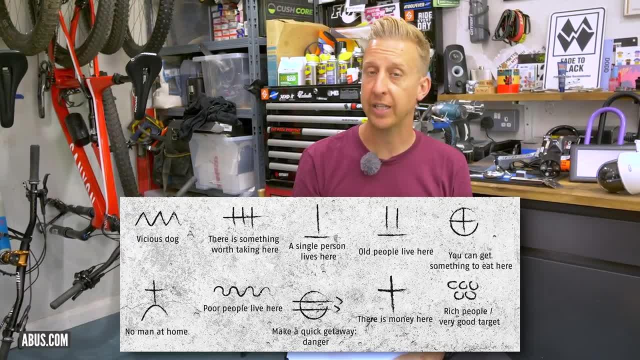 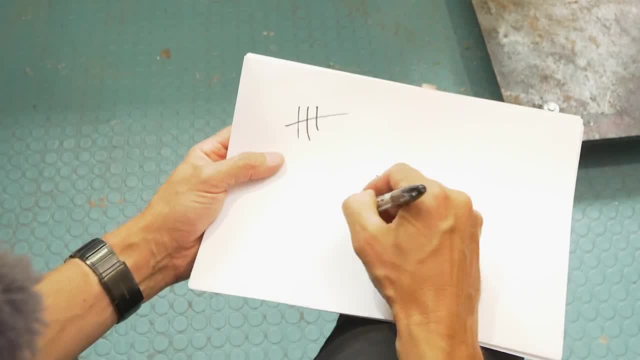 But just to show you a few things, just to show you a few that have been used in the past. If you see any markings like this on the outside of your building, like near the front door or somewhere that could be seen easily, passing by, 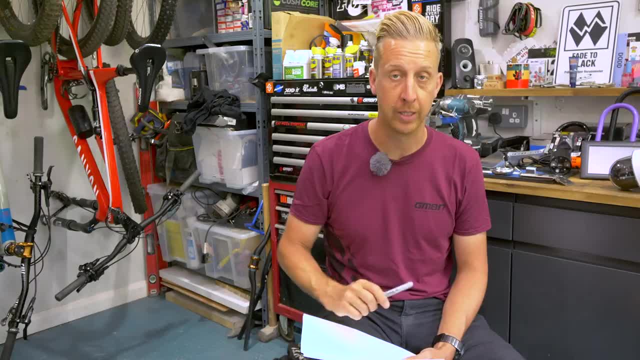 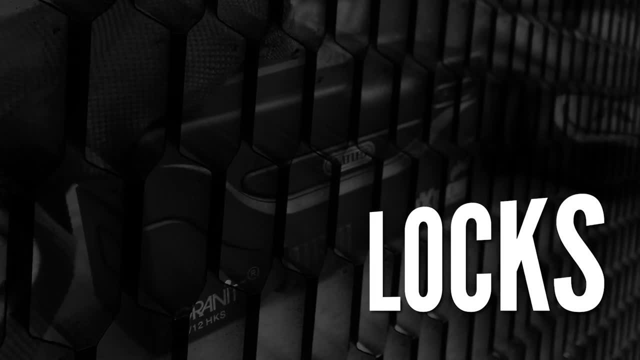 take a photo of them and report them to police and then make sure you erase them and just sort of pay attention, be very vigilant with security. Pretty nasty thing to deal with. Now let's take a look at locks. Now there's a few different styles of locks. 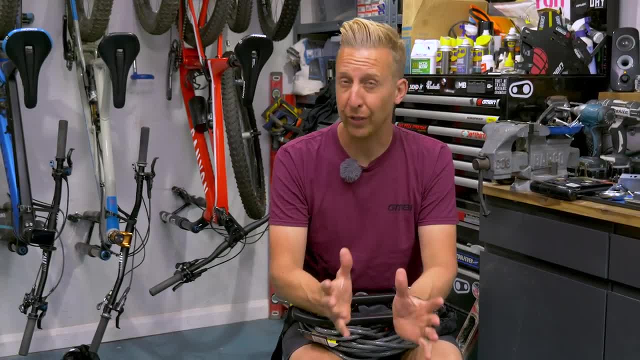 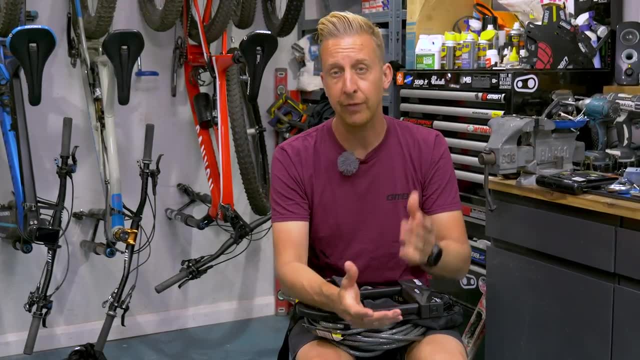 available on the market and there's various different price points. My advice really is to not skimp. Buy the strongest and the heaviest duty locks you possibly can, because really, even though they cost a few hundred quid and it might seem excessive, 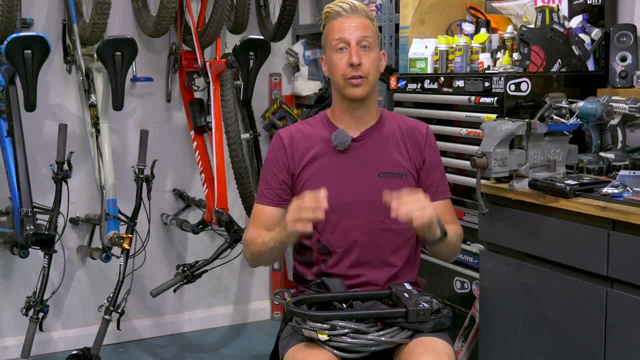 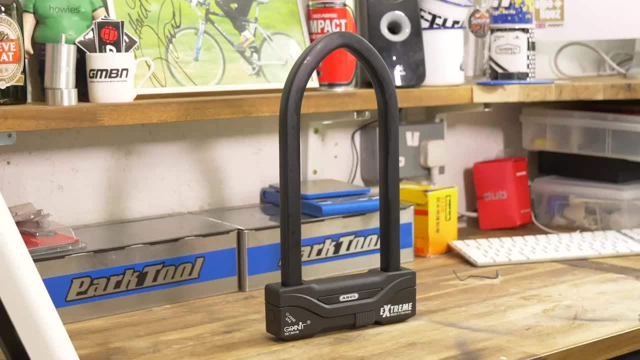 how much is your bike worth? So let's take a look at the three main types of locks you can get and how you might use them at home. So, first up, you're gonna get a U-lock, sometimes called a D-lock. Now, whilst these are incredibly strong, 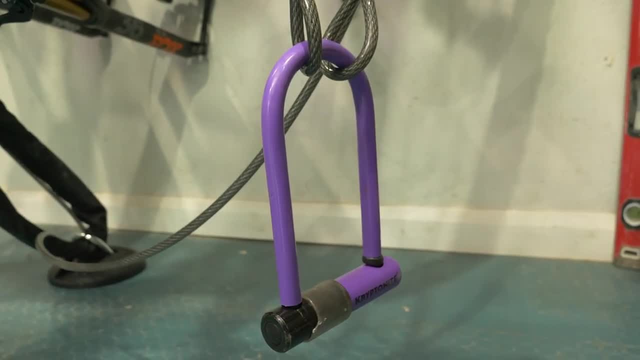 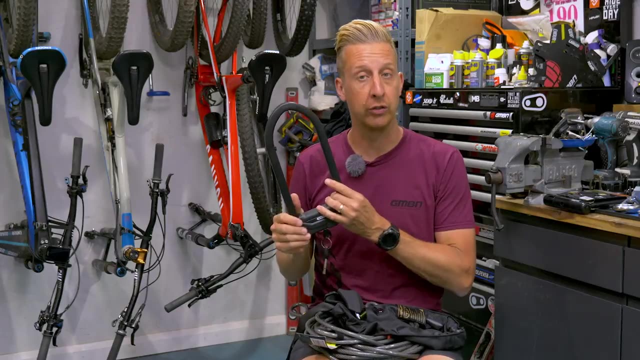 and they're available at various different price points. you may as well take advantage of getting a bigger and stronger chain, A chain lock, for home use, because, whilst these are excellent, they're very limited on how much you can do with them. Great for locking your bike around a lamp post or similar. 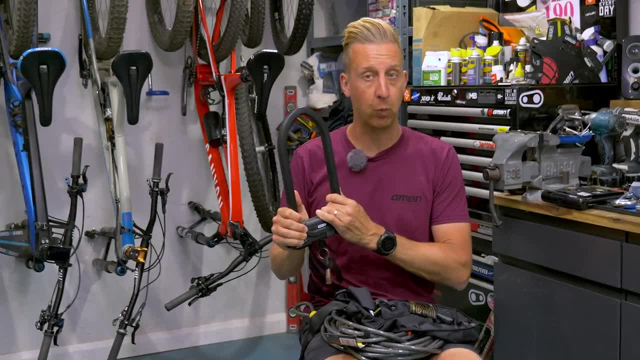 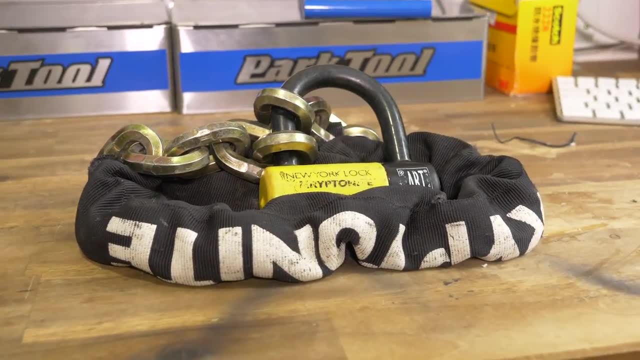 and great for mounting to your bike, but not necessarily the best ones for home. For home, you may as well go all in and get yourself a heavy duty chain lock. There's several brands on the market and there's several styles, prices and options out there. 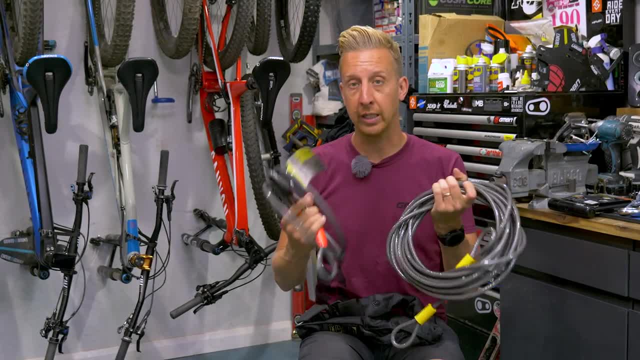 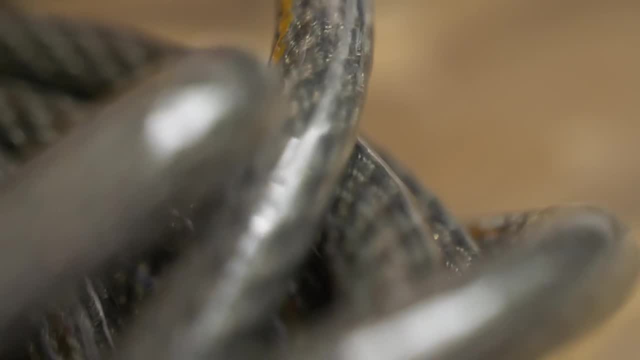 Something else you might want to consider is getting a cable lock in addition. Now, cables are typically extended locks. You shouldn't use these in place of one of the other mentioned locks. These are simply used to go through wheels and frames and, as much as possible, to make nicking your bikes. 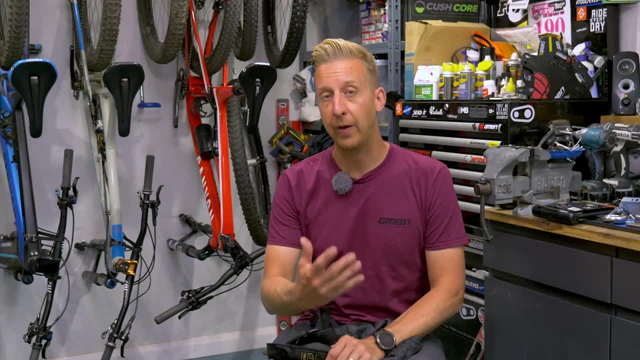 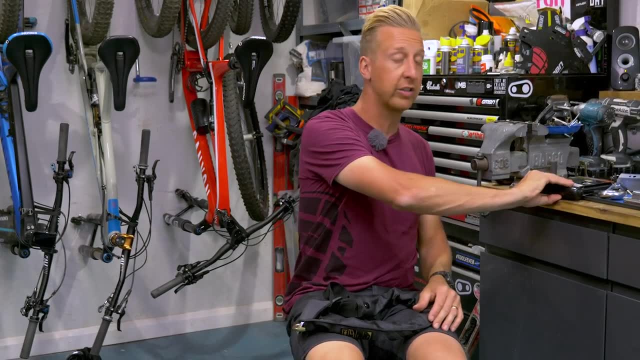 essentially the hardest thing to do Now with locks. there's various different price points and standards of lock depending on which country you're in. In the UK and a lot of Europe we use a thing called Sold Secure. There's a little label you'll find. 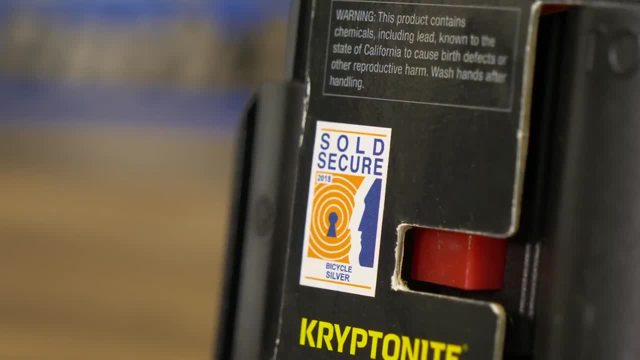 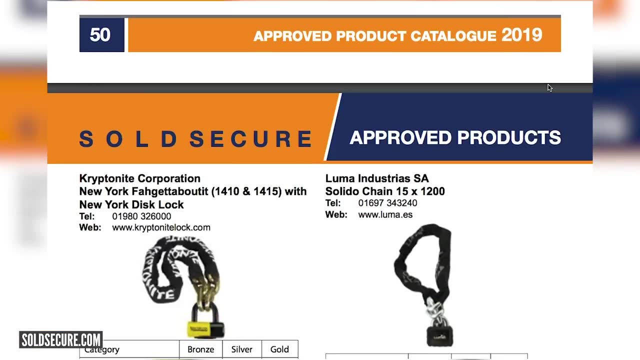 on the back of the packaging and it'll be rated gold, silver or bronze, Bronze being the cheapest and gold being the highest. Now those ratings correlate directly to the value of the bike that you're locking up and how much your insurer may or may not pay out. 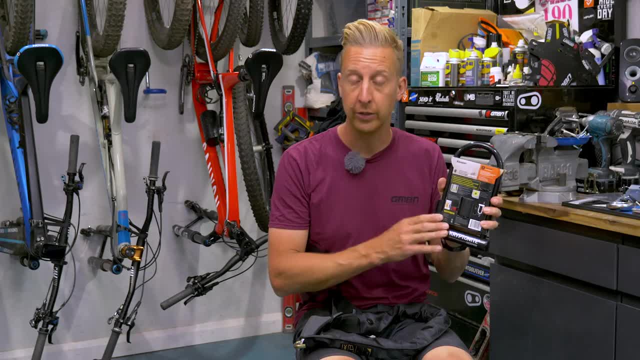 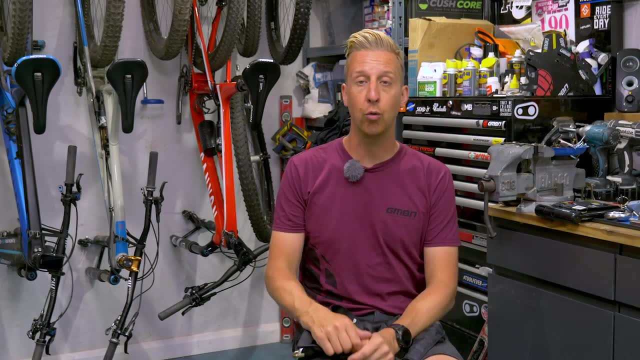 in the event of it being stolen. So it's really important to make sure you correlate that and spend decent money on a lock to protect your bike. But, like I say, all locks are good and all locks are better than no locks. But for home, take advantage of having a heavy duty chain. 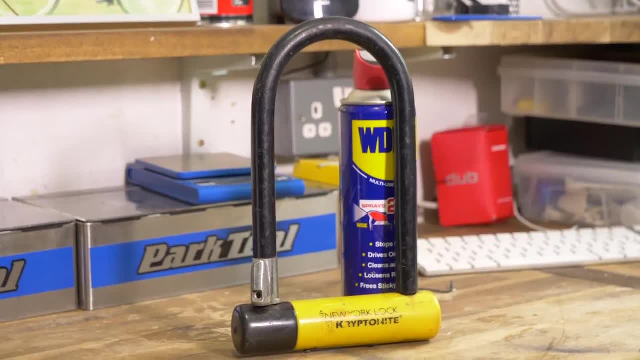 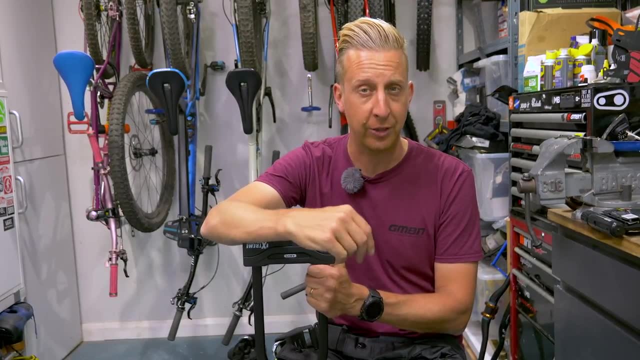 and save the D-locks and the other style locks for out and about. In addition to having the strongest and strongest locks, the strongest and most secure locks, you can make sure that you use them correctly, because how you use them actually is as important. 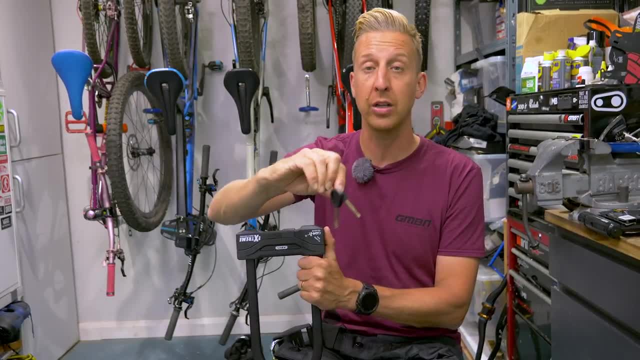 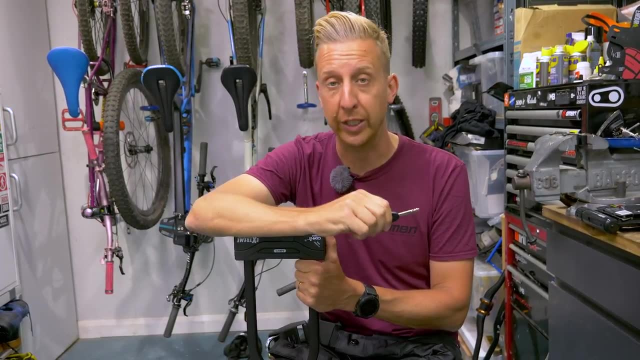 as having a good lock in the first place. Now all locks will come with a master key and at least one spare key, perhaps two or three. Make sure you note down the number of the key and register it if the lock company you're buying from. 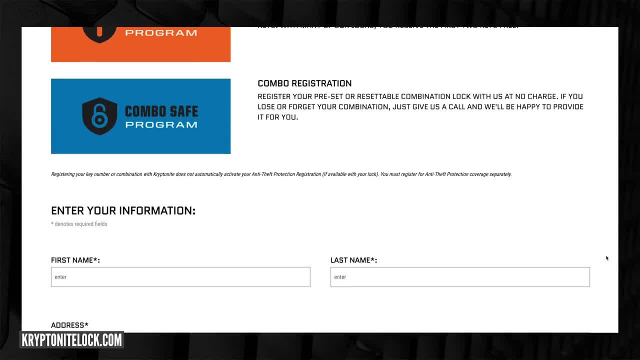 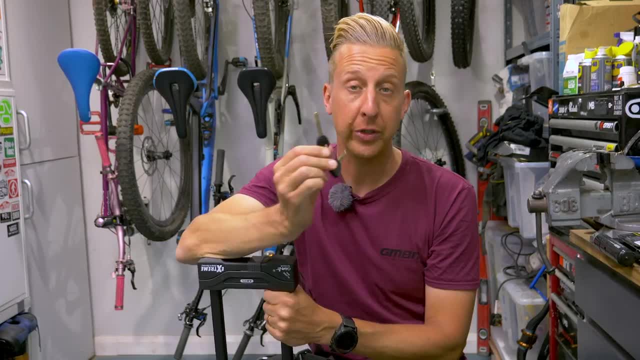 has a way of registering online, because if you do manage to lose the keys, that's the only way you're gonna be able to retrieve it, which is why you need to make a note of the number as well as registering it. Now, make sure you split your keys up as well. 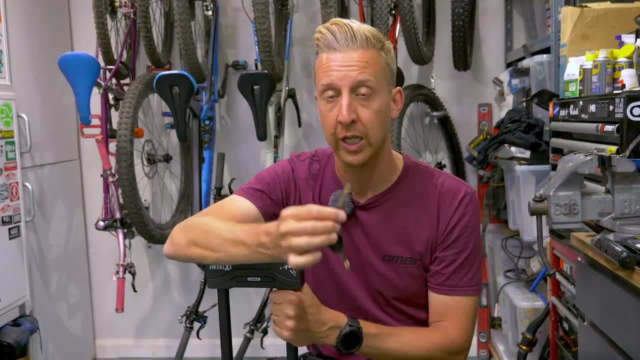 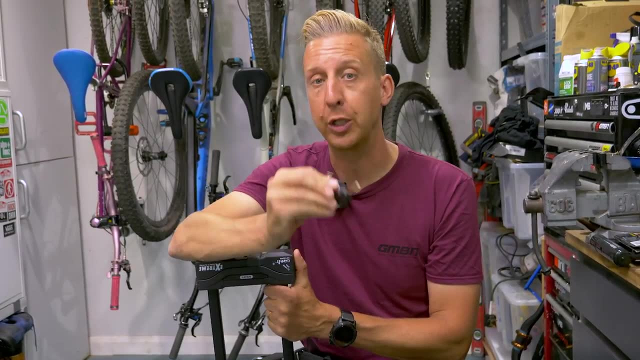 So your day-to-day keys you might have. like myself, I have two or three different locks. I keep those keys together in a secret location that is not in the same room as I keep my bikes, for obvious reasons, And make sure your spare keys are kept somewhere else. 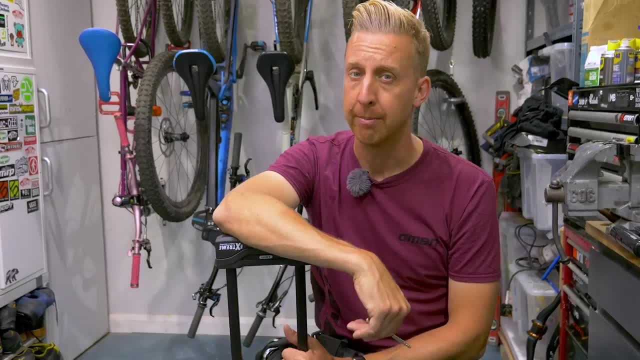 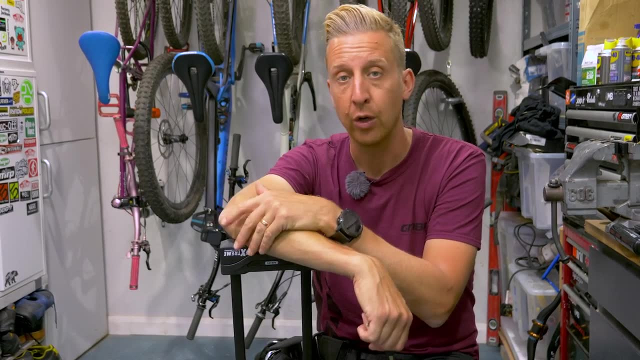 in the house. keep them safe, Preferably in a safe or something like that. Make sure you lock your bike to something immovable. It could be a heavy duty work stand that's bolted to the ground. It could be part of your house. 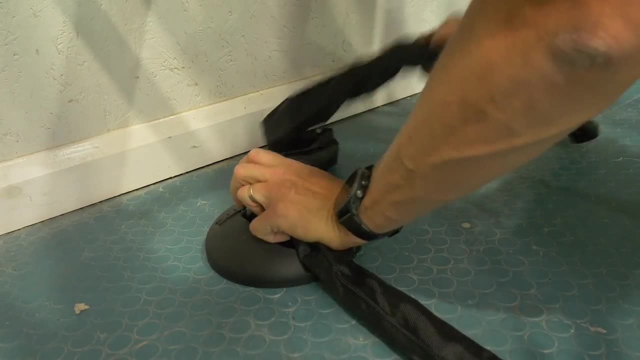 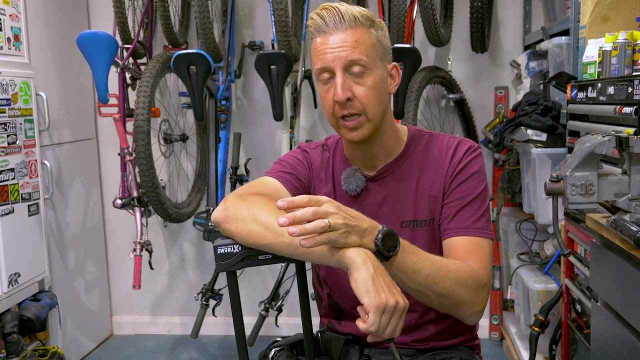 or preferably a ground anchor that's specifically designed, but we're gonna get to that in a minute Now. also, you need to make sure when you do lock your bikes up, you think about a few things, because the way the thieves would be breaking locks. 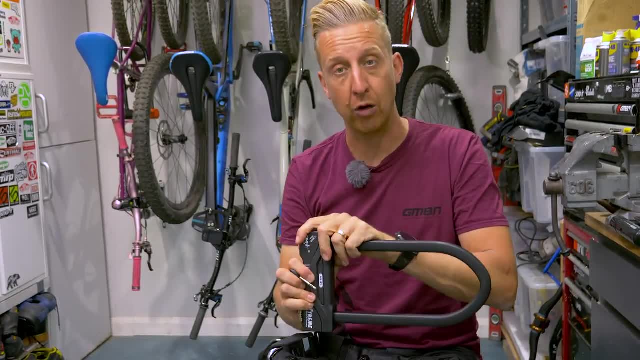 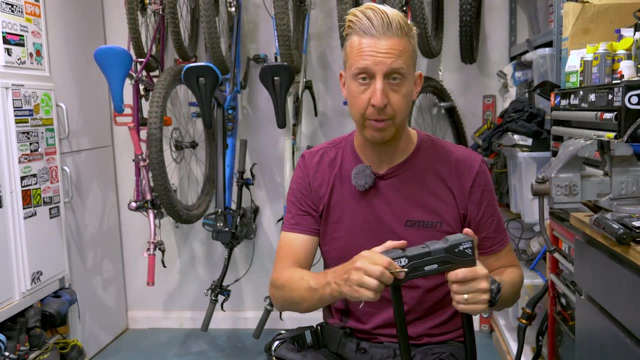 there's various different methods, So sometimes they may freeze the locks and smash them with a hammer. They still have to break the lock at that point. Now, if the locking mechanism is quite close to your frame, it's quite unlikely that they're gonna use that method. 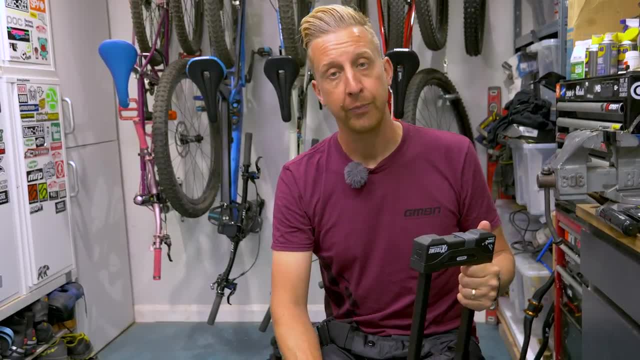 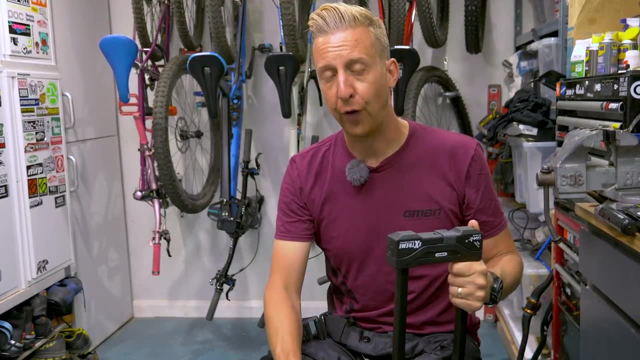 Another method might be to lever the locks open with a big bar, or to use a bottle jack, the sort of jack you get on a car. So try not to give them the space in order to do that. And the final thing, to get around angle grinders. 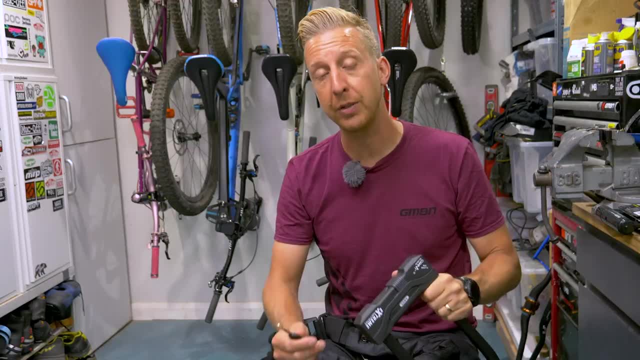 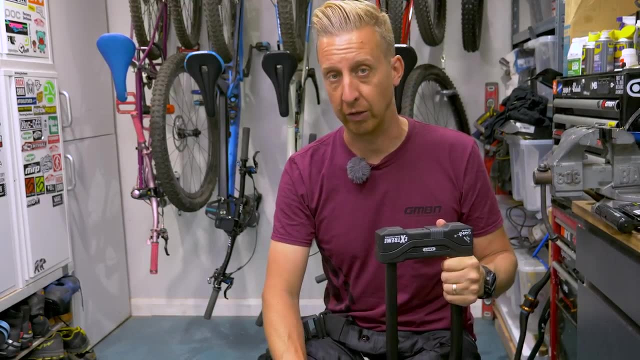 and bolt croppers is to make sure that your locks aren't on the ground or any position where they can get any point of leverage on them. Basically, make it as hard as possible for someone to get to the locks, And the same if you have an anchor point. 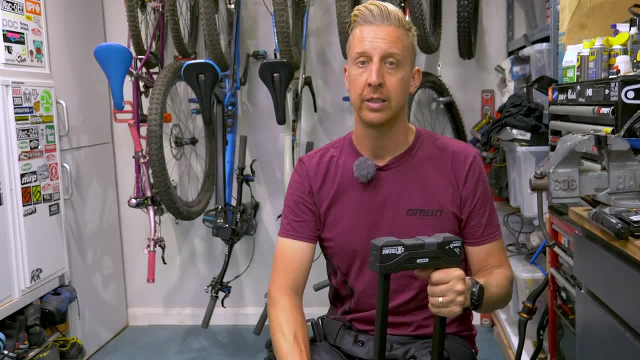 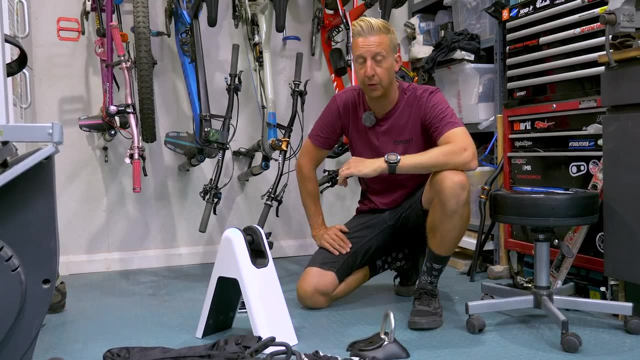 make sure it's tucked away. Don't leave it in the middle of the room where they can work on it. You wanna make this hard for them Now to make sure your locks are in place. your locks are as effective as possible. the best way is to have a dedicated anchor point. 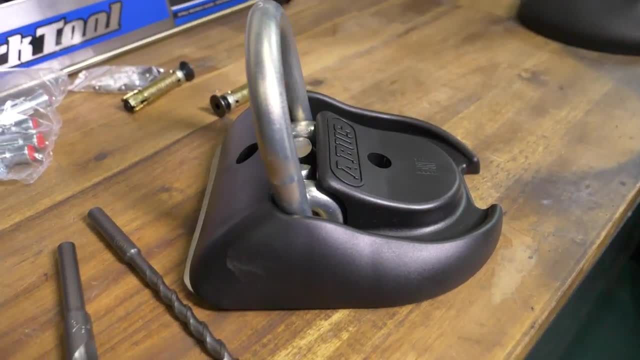 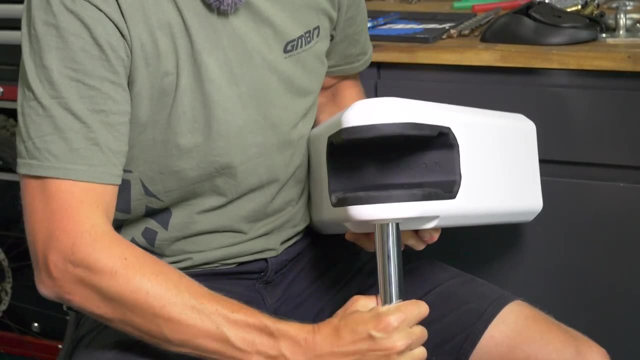 That means having some sort of ground anchor, like one of these, or perhaps a wall anchor. You can mount these on the wall, or you can get a dedicated wall anchor like this one. Your bike actually hangs from this. so if you're limited on space, 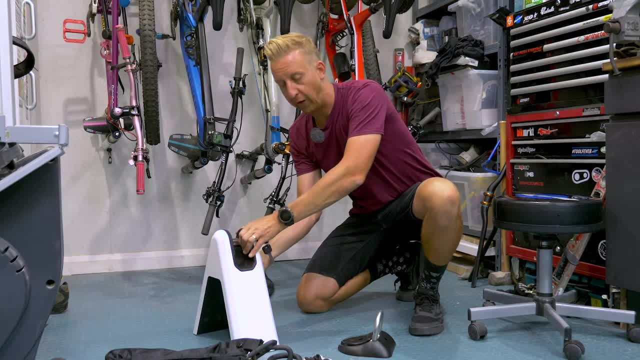 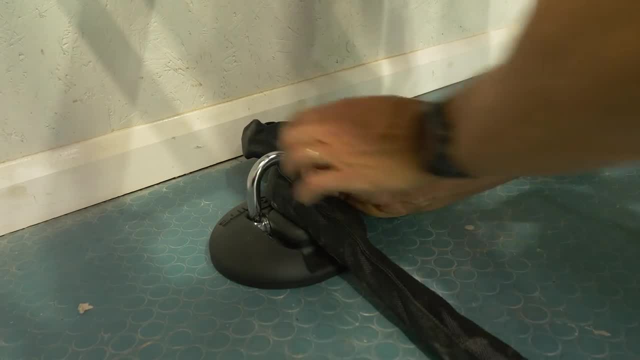 and you want to get your bike out of the way, these can work out quite well. There's various different types on the market. As you can see, I've got a ground anchor in place down here with a big heavy duty gold secure lock on this one. 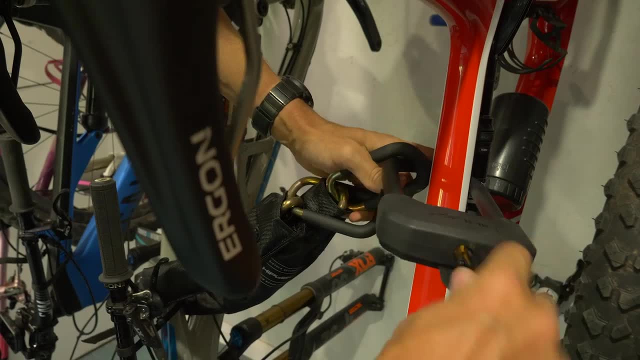 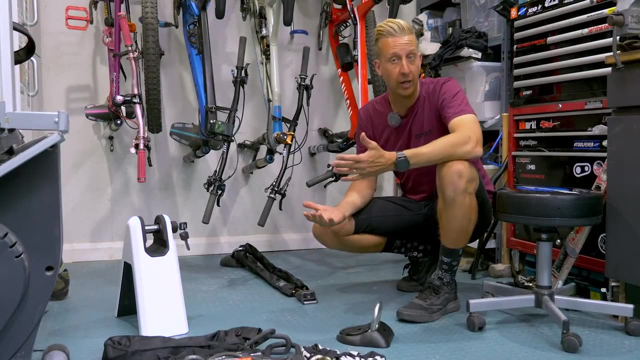 I use this in combination with a whole bunch of other locks, which I basically daisy chain my bikes together and then I lock them to this lock, which is locked to the floor. So ideally there's as many locks in place as possible. 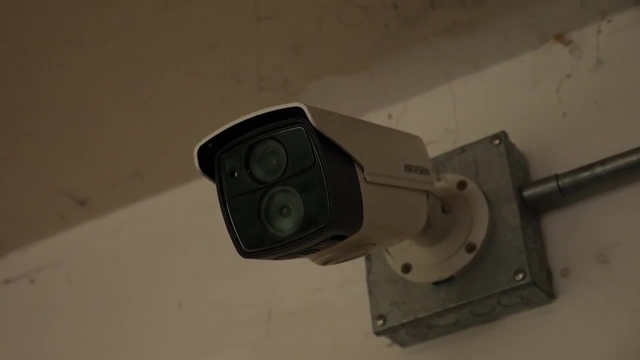 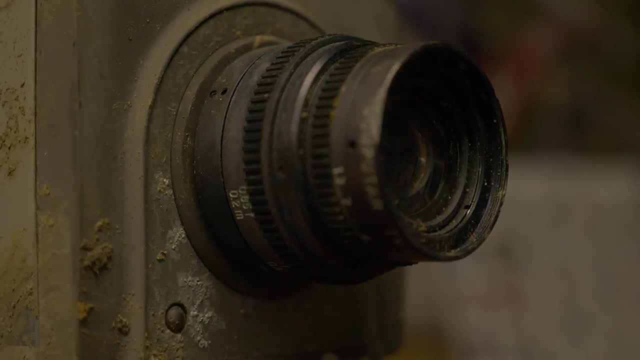 CCTV. now, this might sound like a bit of an extreme option, but if you have a garage or an outbuilding that's separate from your house, then this might be the ideal solution for you, and it's also a very good deterrent. Now there's a lot of different systems available. 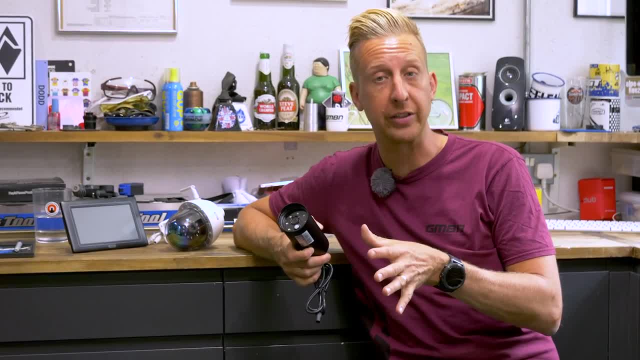 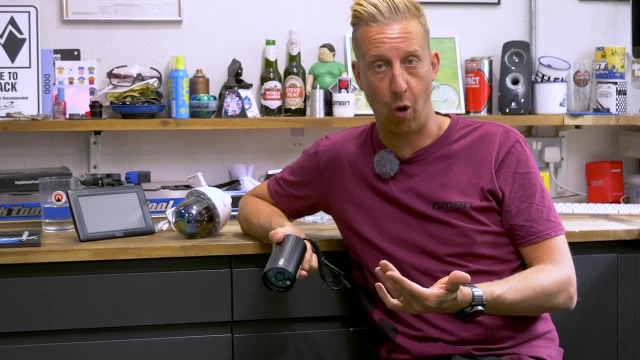 in the market that operate in very different ways. No one system is the best for any one person, so you've got to identify what works best with your property, what it can see, the conditions it's going to operate in and, of course, how usable it is. 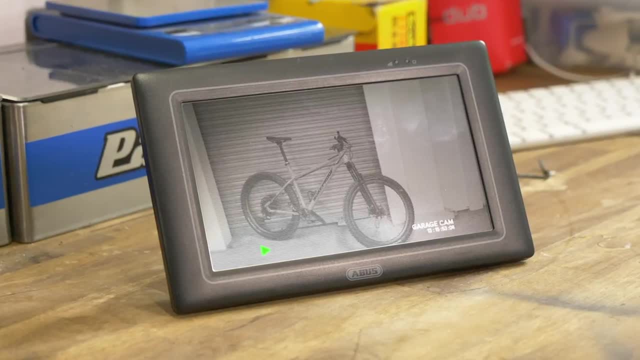 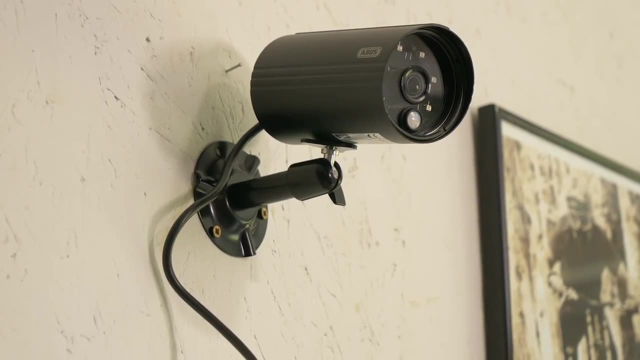 So just for example, these two here: this one has a hard drive that's got a monitor on it and records onto this. It has an encrypted radio signal from the camera to this, So in real time it is filming at any point. 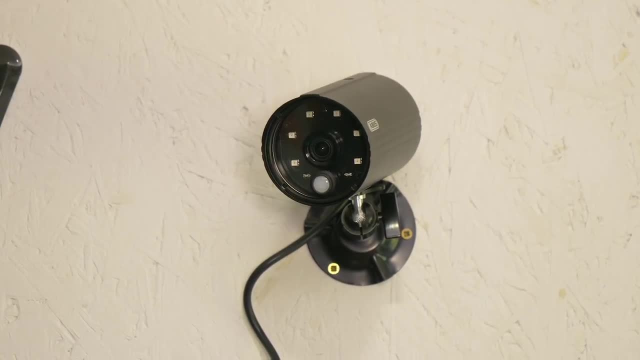 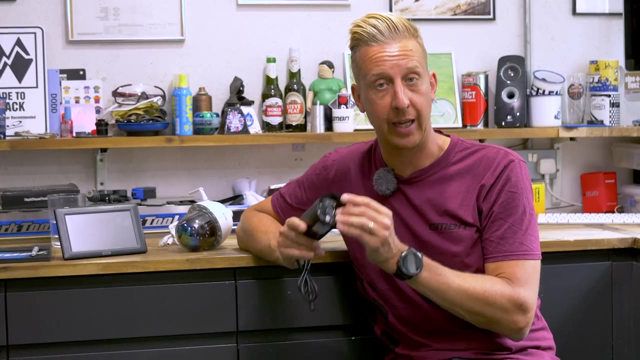 It can loop around so much, like you would have with a dash cam in a car, so you're not having to use new cards all the time And you can also access those remotely from apps. So this is a really cool system. It's an infrared camera on here. 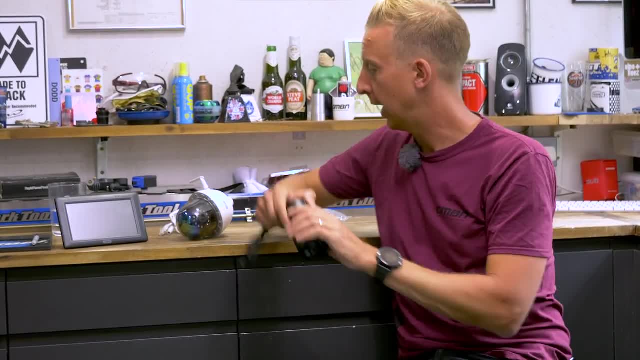 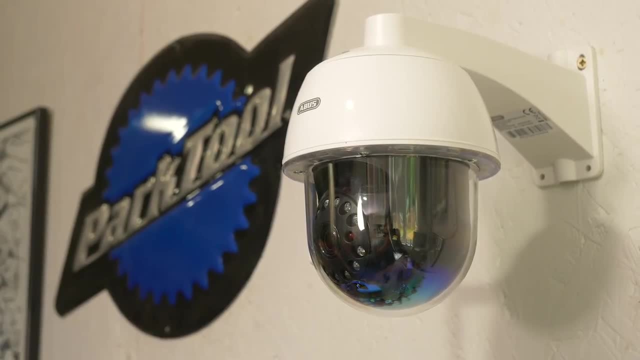 It will work outside, no problem. It's fully waterproof. This is an all-in-one. This is a little bit different. This one works on its own wifi signal or it can go via an own LAN sort of ethernet cable system, depending on how you want to set it up. 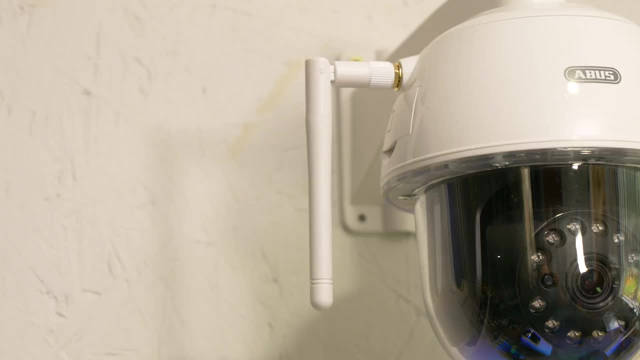 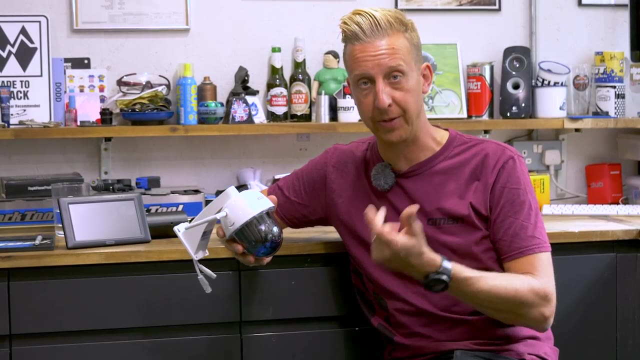 There's a card on the actual camera itself, but also via cloud services and your mobile app you can get all of the information directly to your phone, which means if anything happens, you can screen grab and send that directly to the authorities. 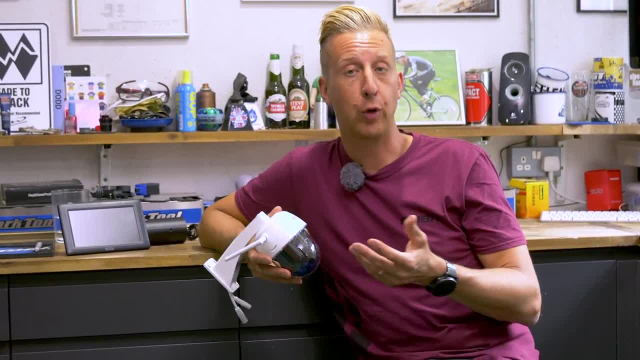 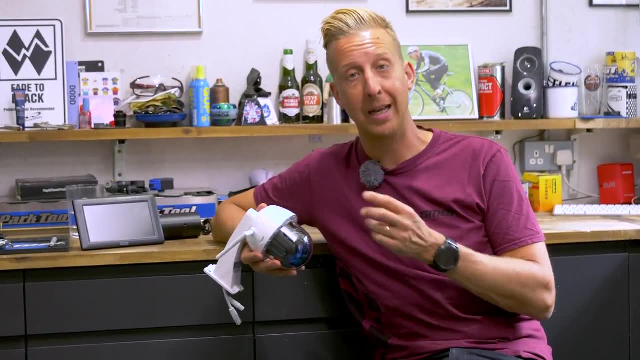 So there are a lot of different systems out there, And of course, you could go the whole hog and have a fully wired system, but something in particular that's definitely worth factoring in is the type of lenses that they operate on and the resolution of them. 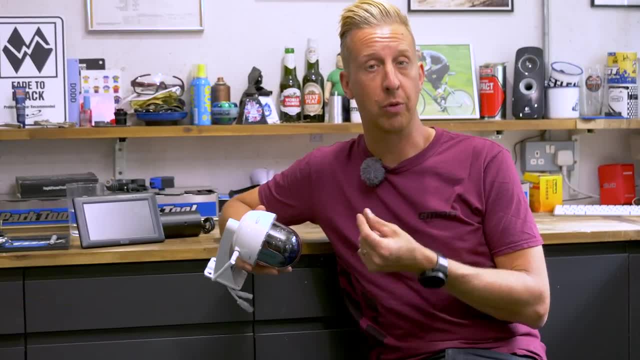 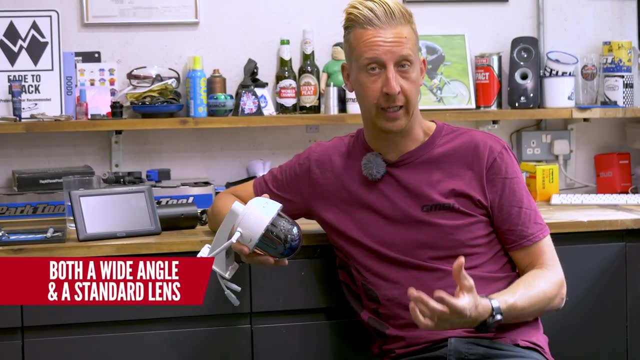 So I would say, at minimum, you want something that's full HD, You want something that's gonna work on infrared so it can see at night, And also you might want something with a wide angle and also a standard angle. The reason for that is a wide angle. 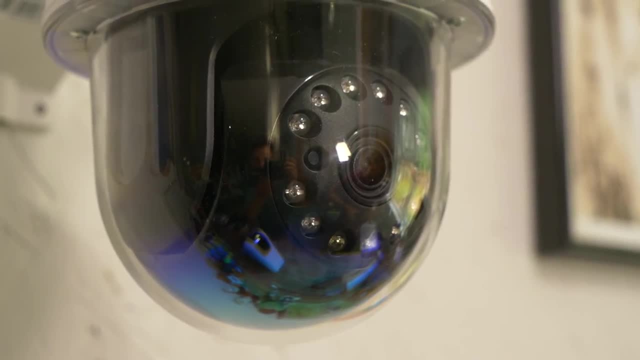 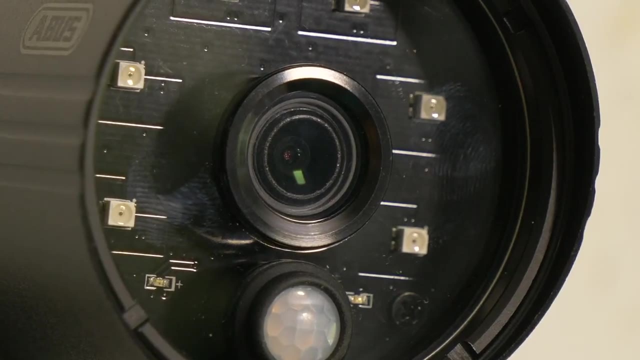 whilst it's very good for seeing a huge area of space, it can be quite hard for facial recognition, Whereas if you had a standard lens aimed at your one weak point, let's just say it was in a garage- the weak point is the door. 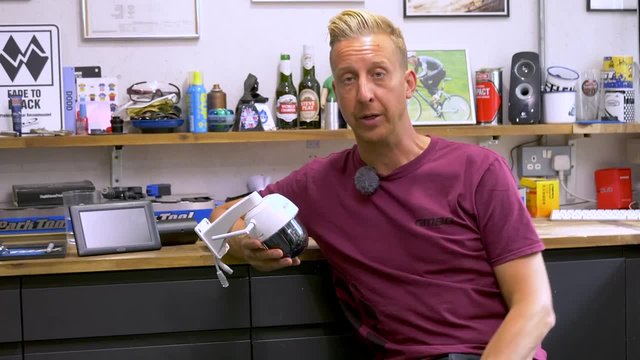 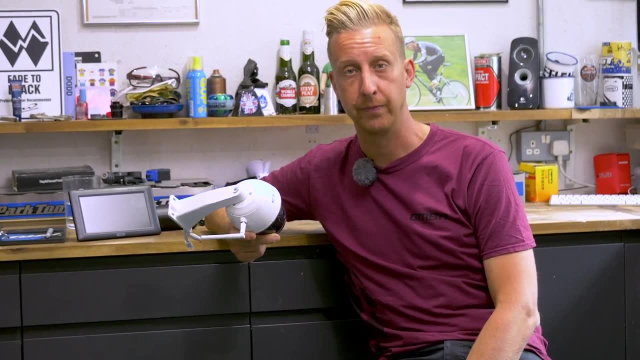 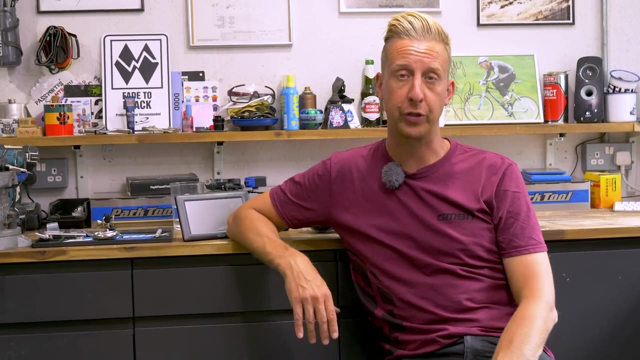 there's more chance you're gonna get a decent resolution still image of the culprit. So just take that into account. Like I said, there's a lot of different systems. Make sure whatever you get works for you. Insurance Now you'd be a madman to not have your bicycles insured. They cost so much money these days you'd really be an idiot not to So definitely look into all the options available to you. There's various bike-specific insurance companies, but more often than not you can add onto your house insurance, But they will be very specific about the policy. 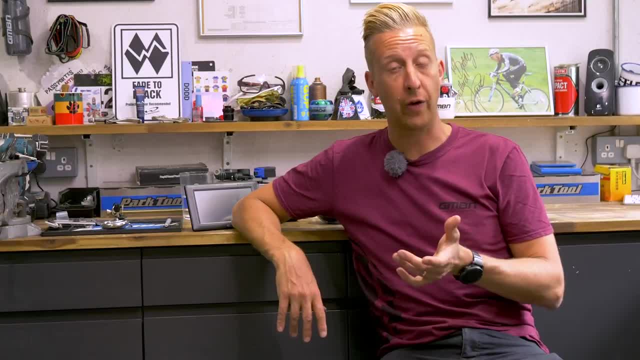 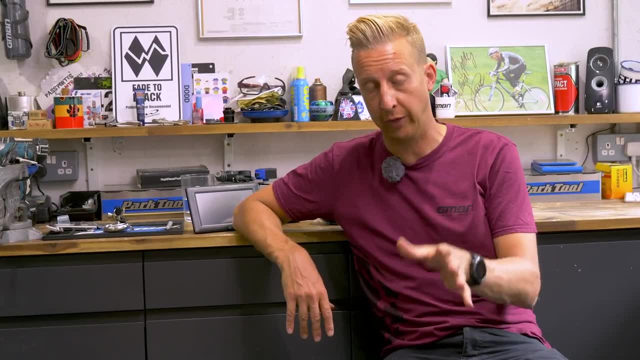 and the payout terms and all that sort of stuff. What you'll normally find is that they will wanna know a description of where your bike is locked. They'll wanna know the details of the building it's in, if it has windows, all that sort of stuff. 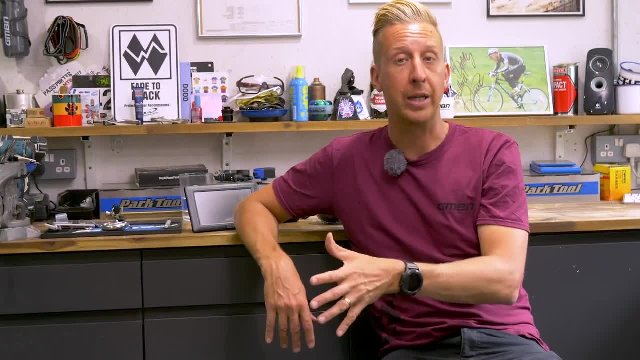 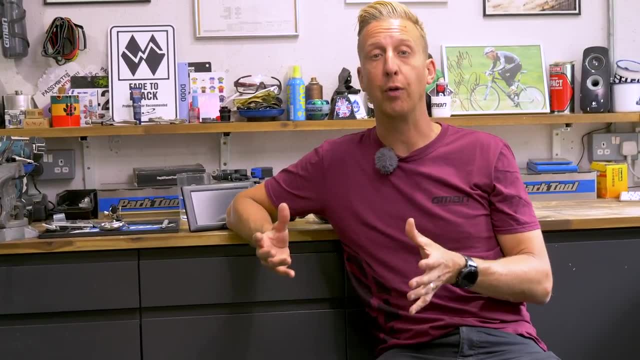 And if you have a ground anchor, they'll want a photo of the ground anchor being used. They'll wanna see what sort of locks you've got. They'll want the serial numbers and things like that of your bikes. So make sure you have all of that information to hand. 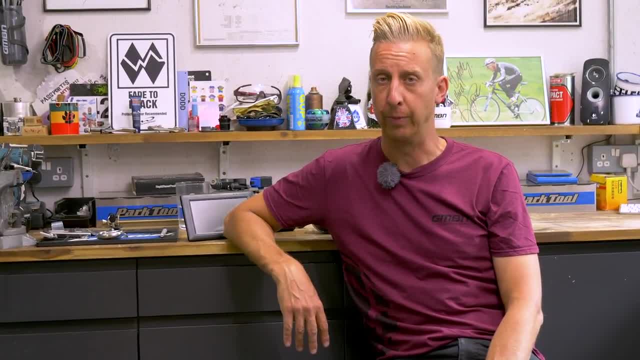 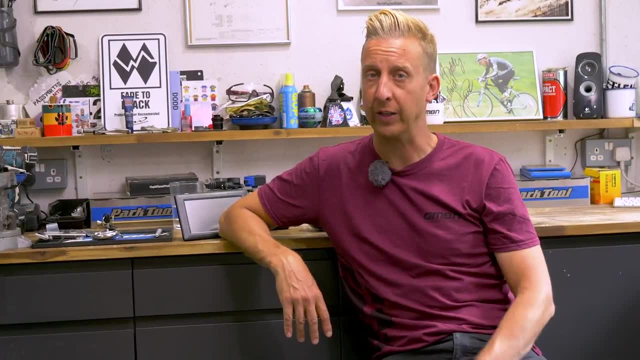 to get the best possible quotes And definitely shop around as well, because it's pretty unlikely the first place you ring is gonna give you the most competitive quote. but I can assure you it's definitely worth having decent insurance for your bikes. It might be really cool in the comments below. 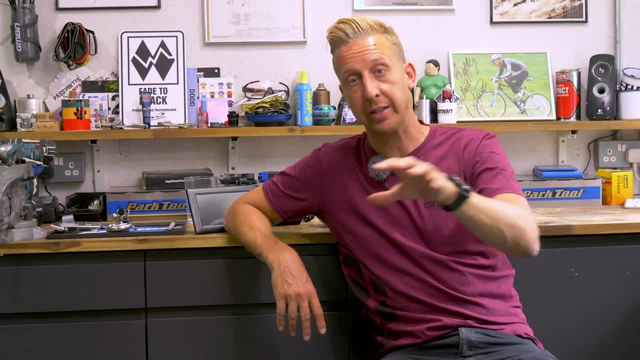 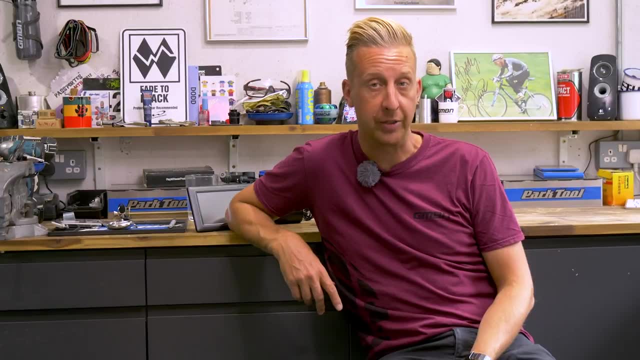 to help all your other viewers out. If anyone can add any advice on various different countries like the US, or maybe in Germany or wherever you're watching from what sort of situations and what insurance companies have worked best for you. Let's try and make this a sort of a group sort of thing. 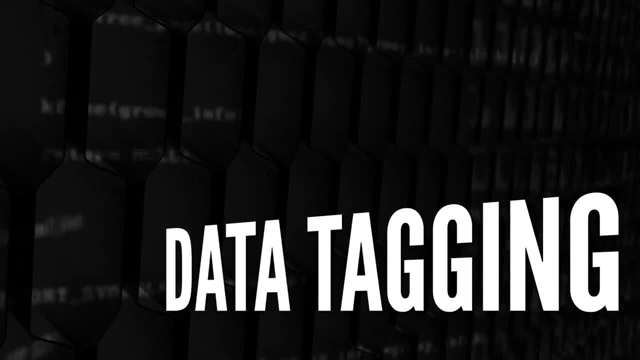 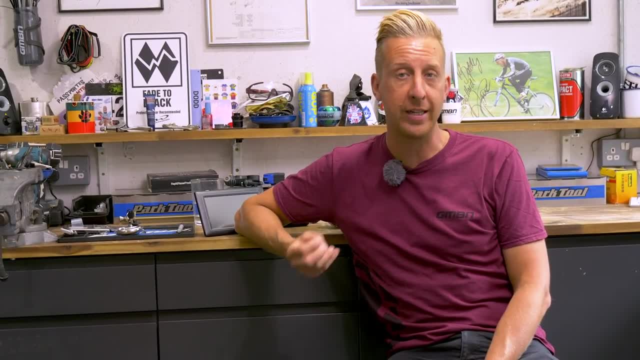 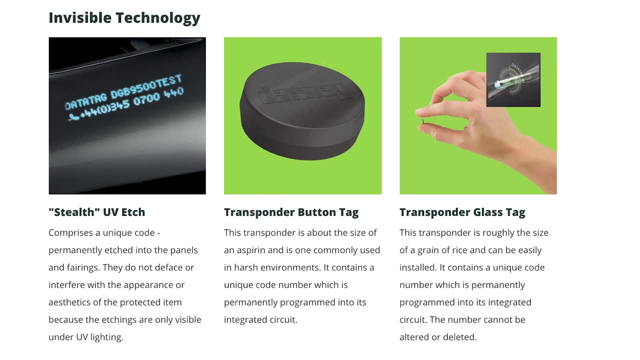 so everyone helps each other. Let us know in the comments underneath. Now in Europe we have a system available called DataTag. It's essentially a forensic marking system for your bike. Once it's marked, it can be tracked virtually anywhere. It dramatically reduces the chances of you losing your bike. if it is stolen, They can be retrieved, And it's one of the ones that's actually enforced by a lot of insurance companies. They will quite often only insure you if you have DataTag in place. That's certainly for UK and Europe. 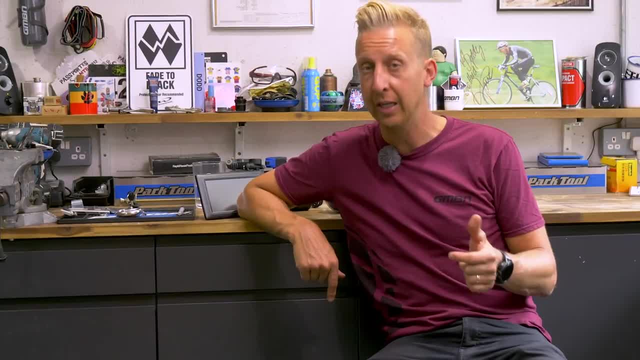 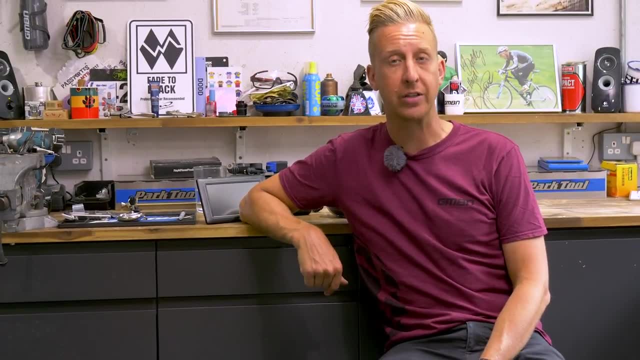 I know in the US there's a similar GPS system called Sherlock. Again, there's different options available to you, But definitely check out all of the systems. At the end of the day, you want to make it as hard as possible to have your bike nicked. 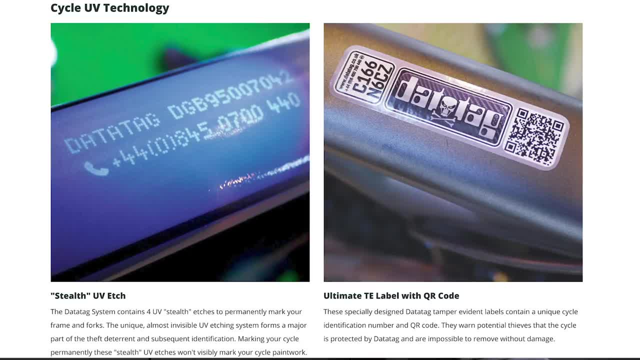 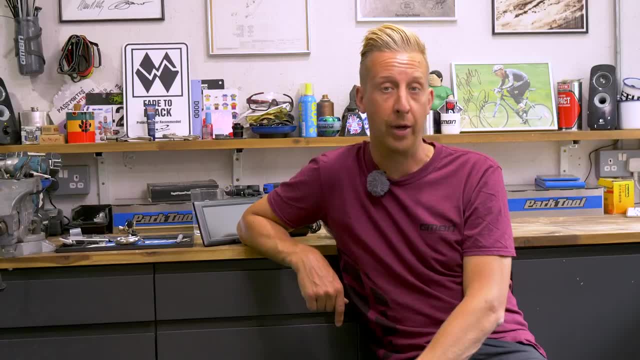 And they come with markings for the bike that display that it's got a DataTag system installed to it, and they're tamper-proof as well, And those alone can be a deterrent from having your bike nicked. So definitely look into things like that. 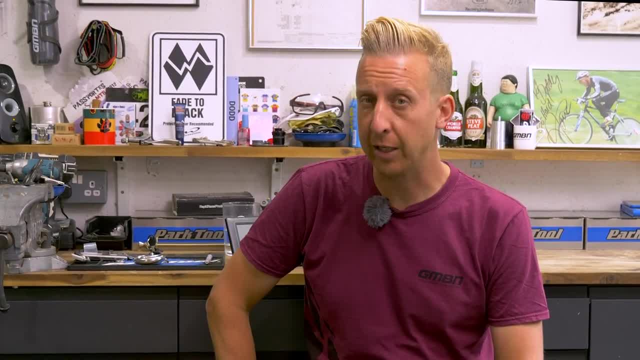 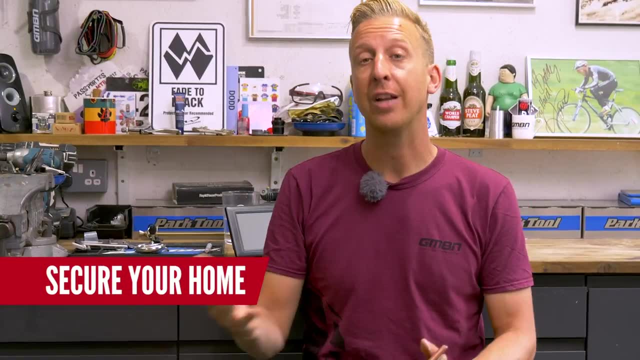 Now you can do everything we've mentioned so far, and still you have to apply some common sense to make sure your bike stays safe. So, firstly, you need to make sure that your entrance to your house is secure, Because if that's not secure, people can still get in. 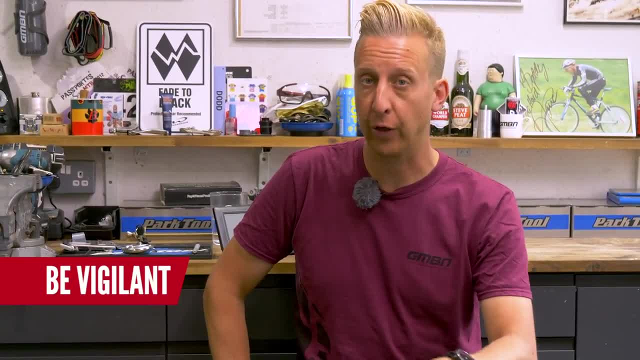 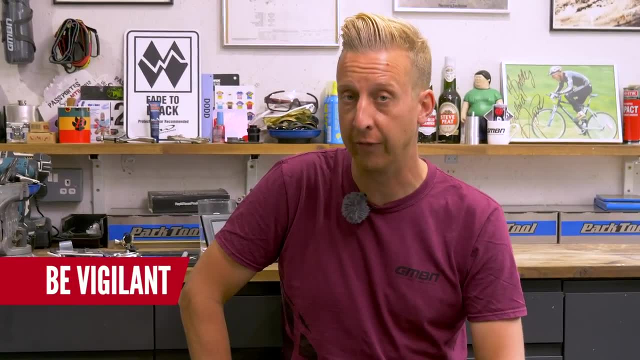 And likewise, if you're aware that there are people around that can identify that you're on a good bike, when you return home, maybe do a lap, go around the block. Don't always return straight into your house so they know where you live. 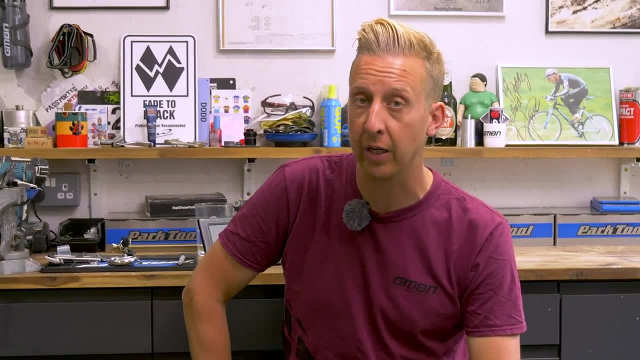 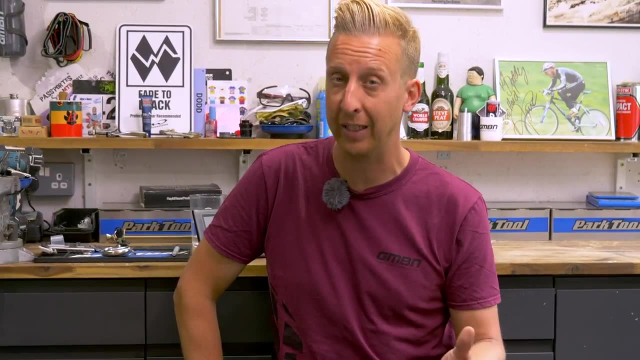 The same applies if you're leaving, maybe, a trail center, when you come home from riding and you notice anyone following you. Although this might be a super rare occasion where you might not have even heard of this happening, it does happen, So just be vigilant about this sort of stuff. 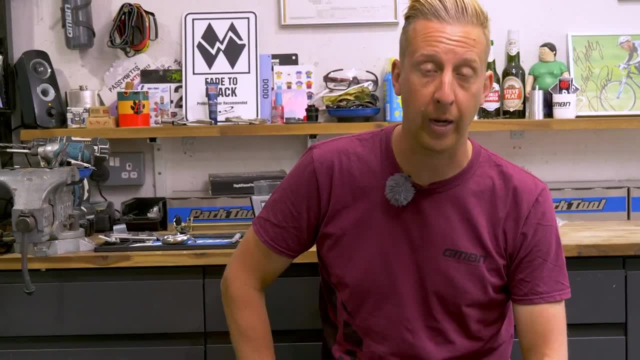 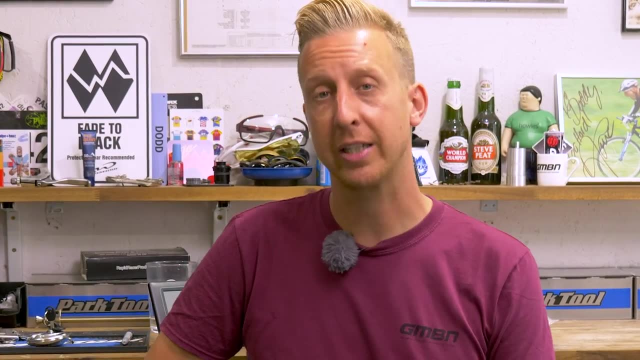 The same applies as to when you're putting a bike in the car, perhaps on your driveway, or unpacking your bike. You never know who's watching, so just take care with that sort of thing. You might live in a perfectly nice neighborhood. 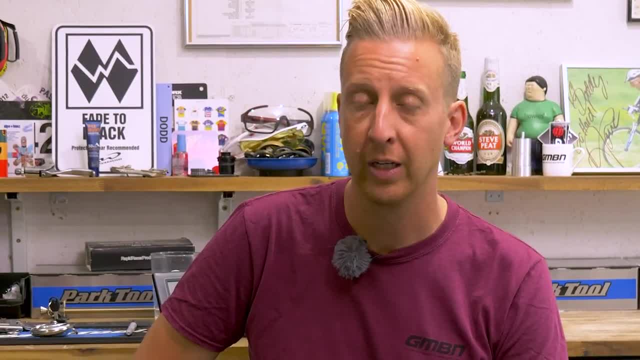 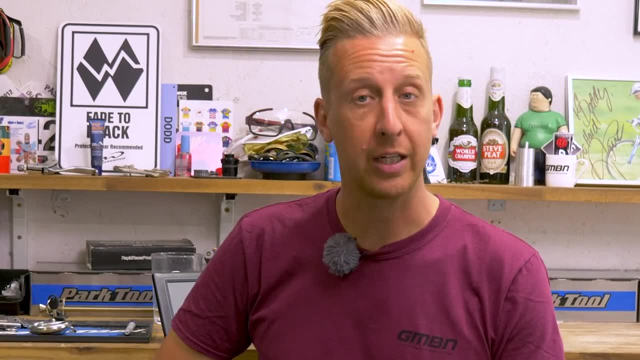 but you can still get dodgy people driving past. so just take note of the house number you lived in. So be very careful with that sort of stuff. Now, another common sense thing is: take note of the frame number of your bike. You'd be surprised how few people actually do this. 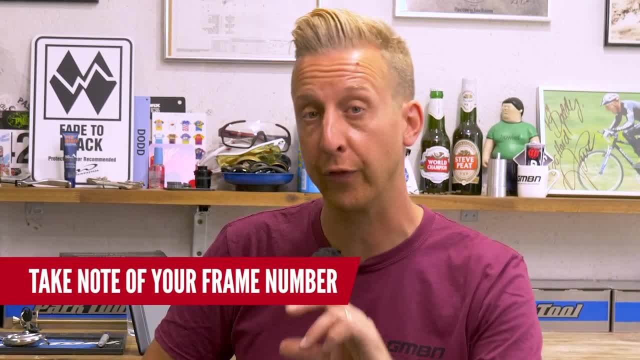 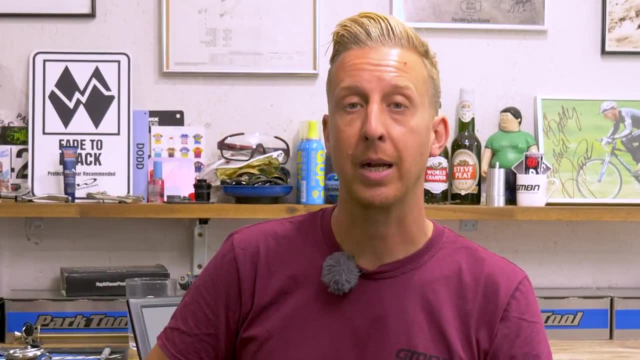 Whenever you get a bike, there is a frame number on the frame. It's sometimes, and quite often, on the bottom bracket shell, but it can be inside the rear dropouts. There's a number of different locations. it can be on a frame and it's completely unique to your bike. 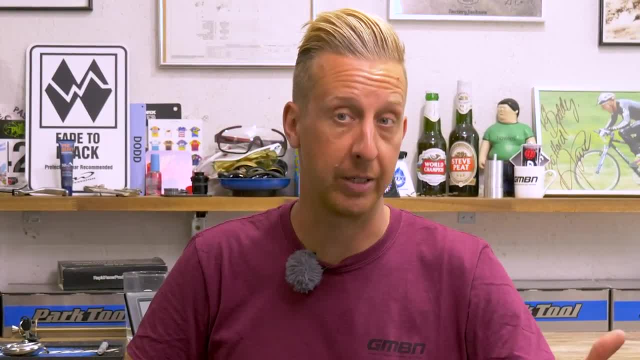 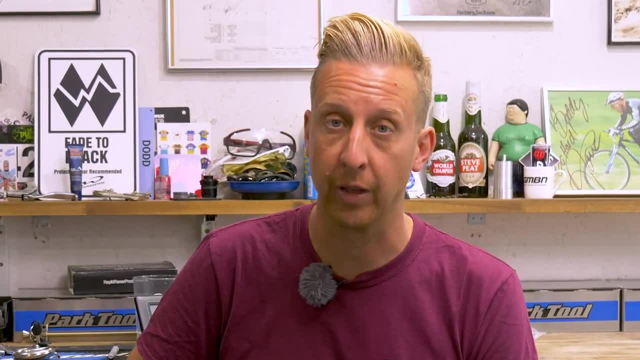 So that means your bike can be traced if the bike is found and it has been stolen, for example, and you will need that number for insurance purposes, and you will also need it if your bike does go missing, to report to the police. So please make sure you note down your frame number. 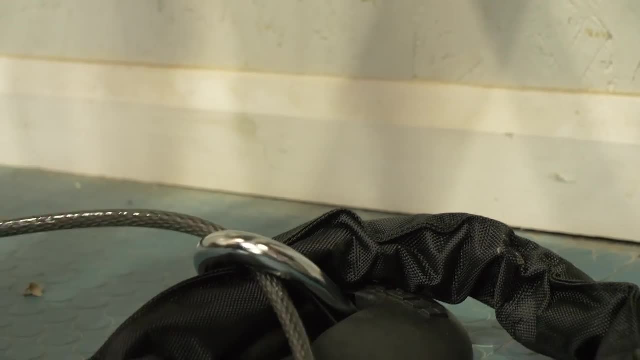 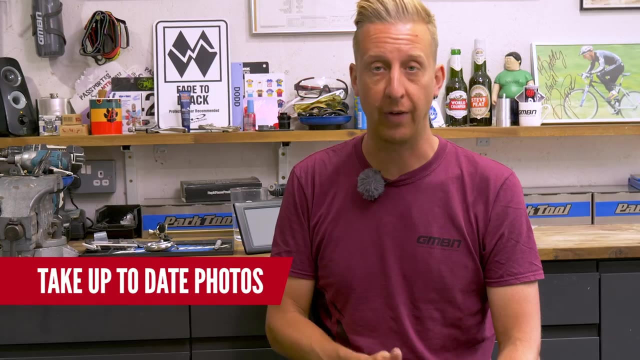 So when you have a good setup, you've got your ground anchors, you've got your bikes daisy chained together and locked to the anchor. take some photo evidence of that and also make sure you have up to date photos of all of your bikes if you have more than one. 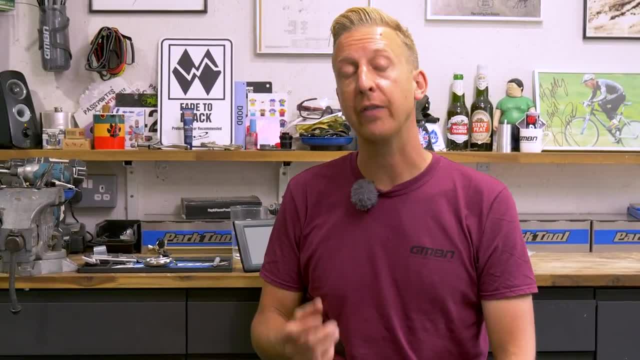 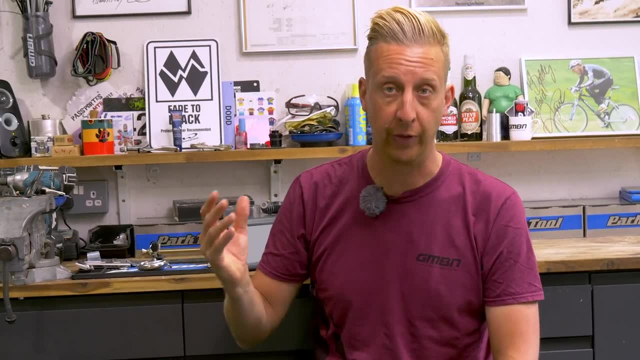 or of your bike, if you only have one. The reason for that is, if it does go missing straight away, you have an image you can share on social media, or you can share with the police or anyone relevant to helping you retrieve your bike. But whilst you're at it, make sure you turn off. 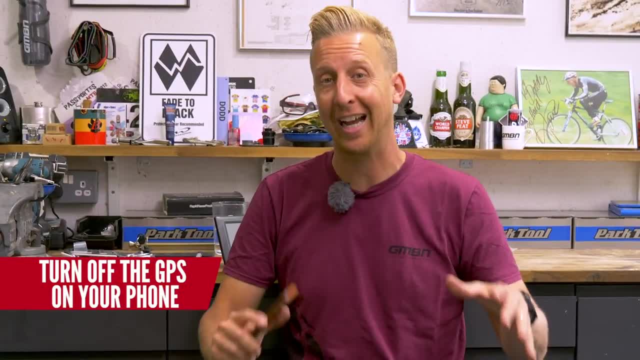 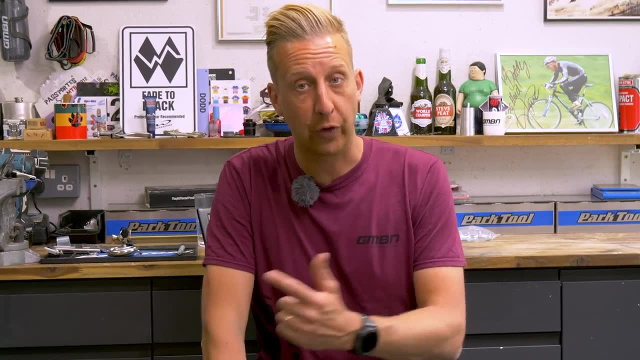 your GPS on your phone if you're taking pictures of your bike at your property. So any of you that take photos for Bike Cave or any of you that take photos for Bike Vault on the Dirt Shed Show, make sure you turn off location services on your phone when you use the camera. 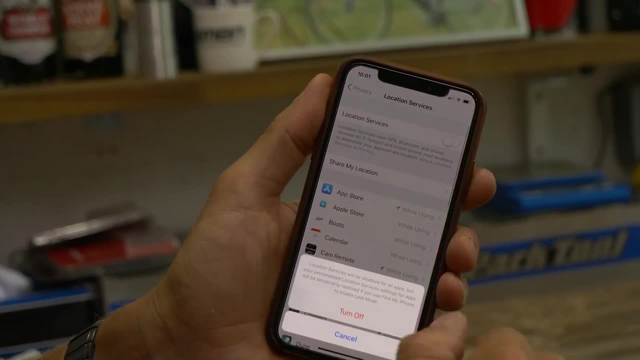 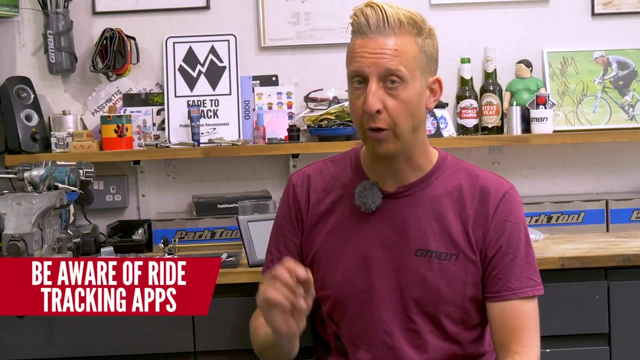 or at least disable them, just for your camera. And the same goes if you use Strava or any sort of ride tracking apps that are available out there. there's a lot of them. make sure that you don't use it from your front door. 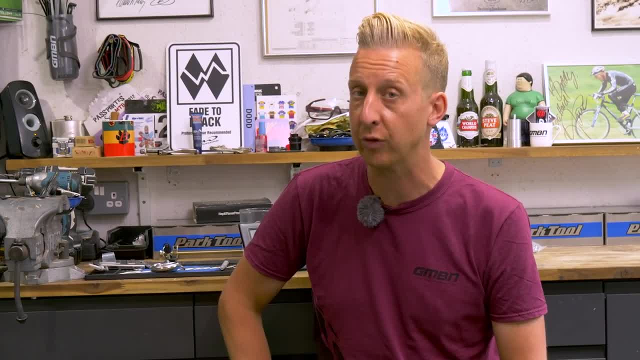 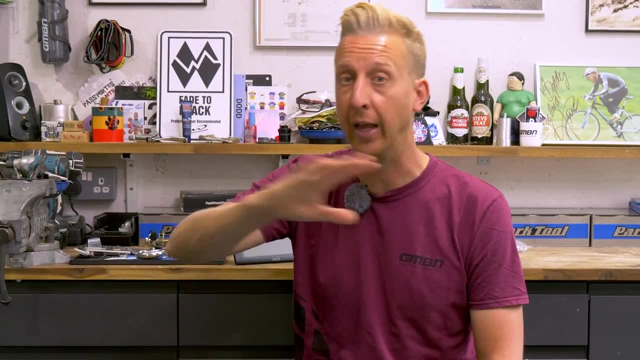 You can set up privacy zones on Strava, but I would still not completely trust that I would go for a ride first, then start your official ride tracking and then return at that point and then return home. You really don't want any way that you can be traced. 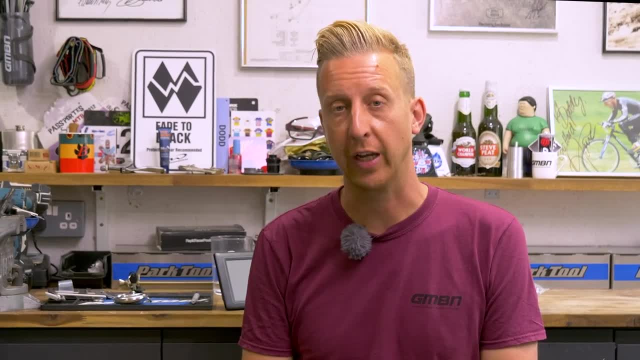 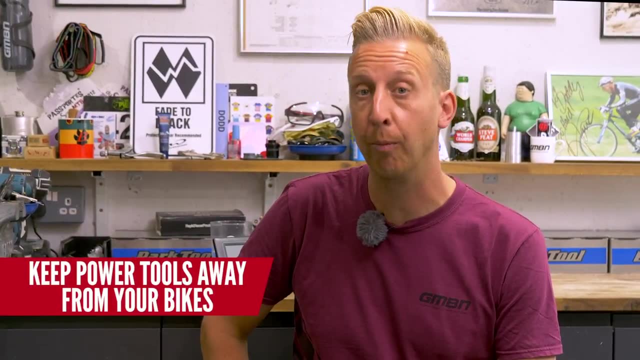 back to where you live. Now, just a few last little things to say. If you have heavy duty power tools in your workshop, for example, it's a good idea to keep them locked away, or perhaps in a different location from where you lock your bikes, just in the event that something bad 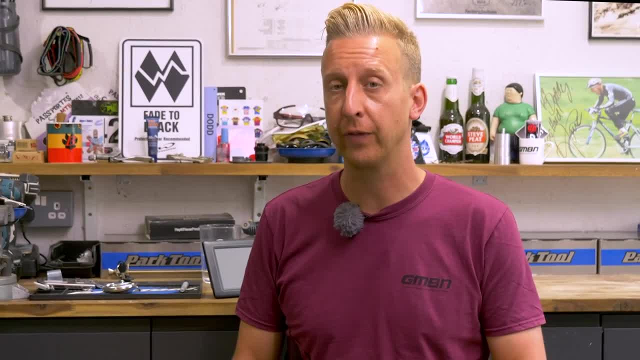 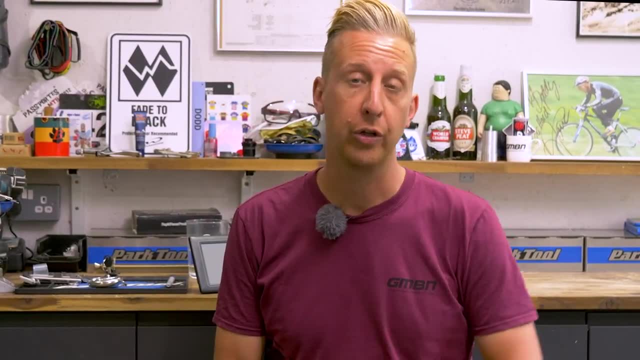 could happen. If you have any of those sort of feelings about any stuff, use your instincts. Close your blinds at night so people can't see in. Make sure you've got cages over the windows. Lock your doors, use CCTV, have alarms, have anchor points.